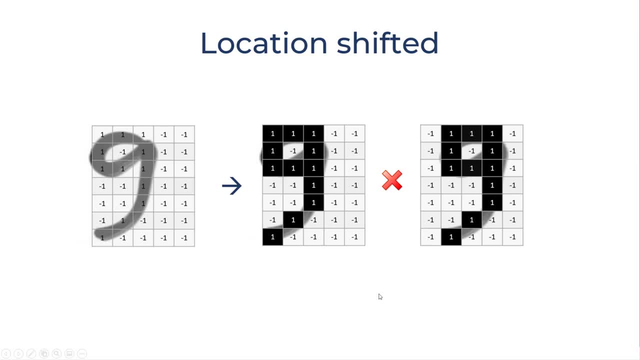 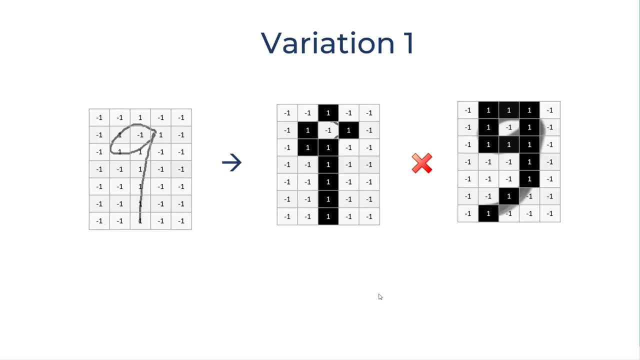 match with our original number, grid and computer will not be able to recognize that this is number 9.. There could be a variation, since it is a handwritten digit. There could be variation in how you write it, which will change the two dimensional representation of numbers and again you will not be able to match it with the original. 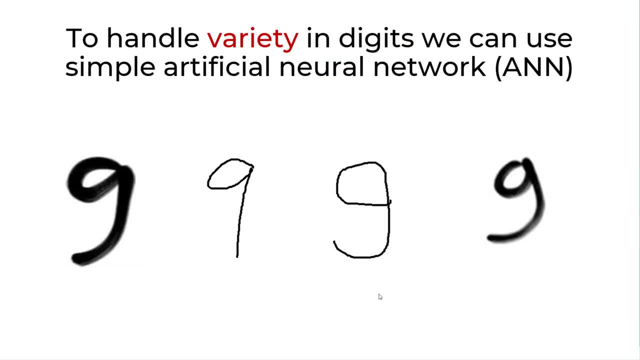 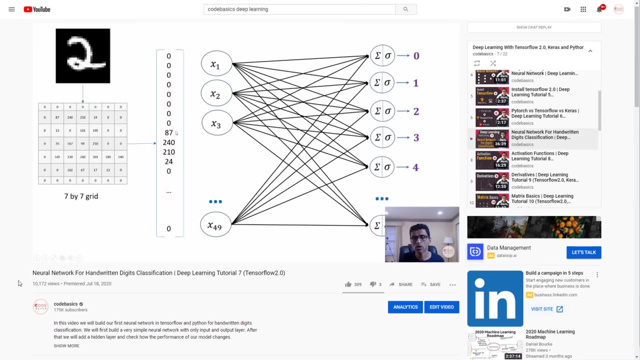 grid. So we use artificial neural network for this kind of case to handle the variety In this deep learning series. we have already looked at the application of artificial neural network. We have already looked at the application of artificial neural network video on handwritten digit recognition. If you have not seen that. 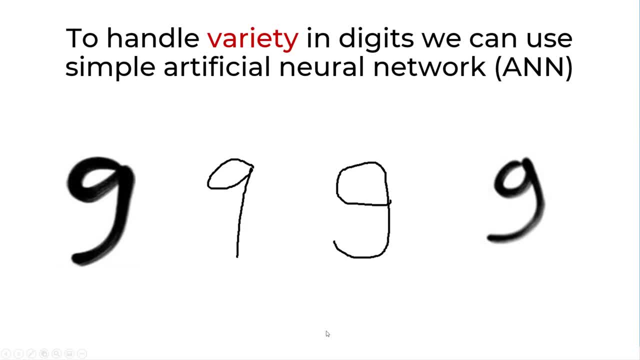 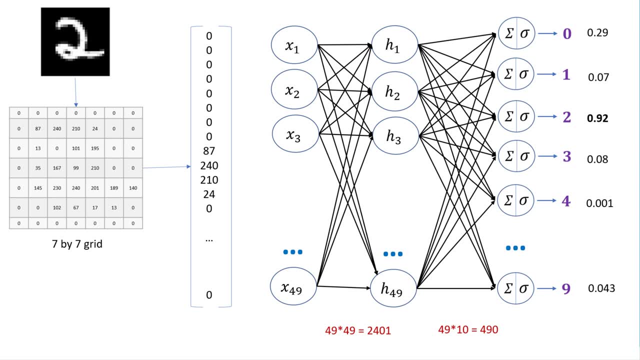 video. please make sure you see it so that your fundamentals on artificial neural networks are clear, In that we created a one dimensional array by flattening the two dimensional representation of our handwritten digit number, and then we build a neural network with one hidden layer and then we create a neural network with one hidden layer. This neural network will work. 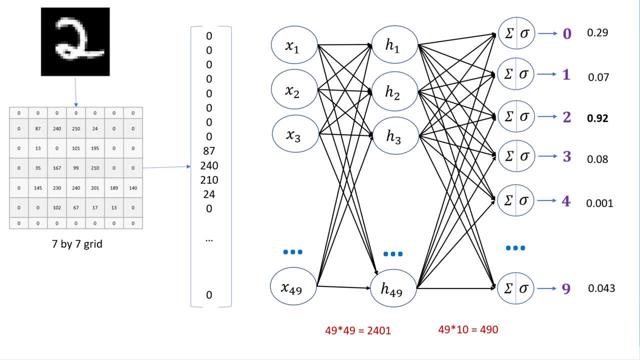 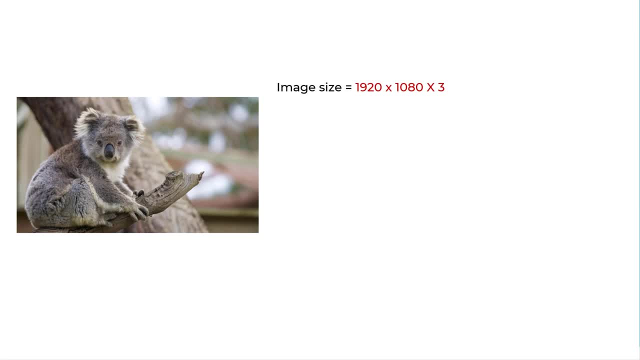 ok for a simple image like handwritten digit, But when you have a bigger image, let's say this little cute looking koala. The image size is 1920 by 1080.. We have three as RGB channel here: One for red, green and blue. In this case, the first layer, neuron itself. 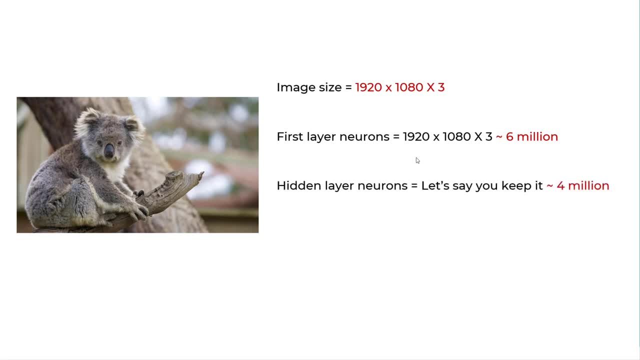 will be six million. If you have, let's say, hidden layer with four million neurons, then you are talking about 24 million weights to be calculated just between the input and hidden layer. And remember, deep neural networks have many hidden layers, So this can go easily. 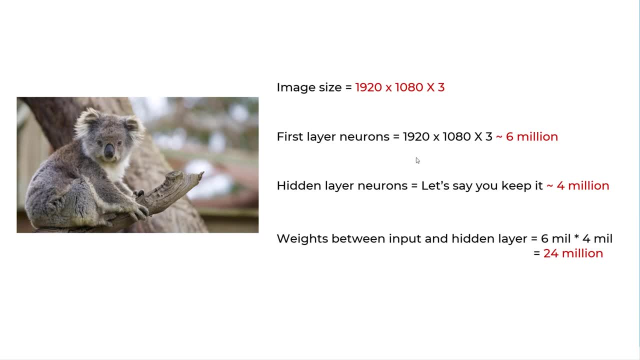 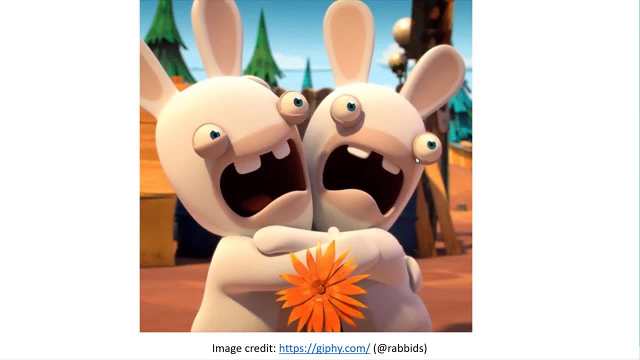 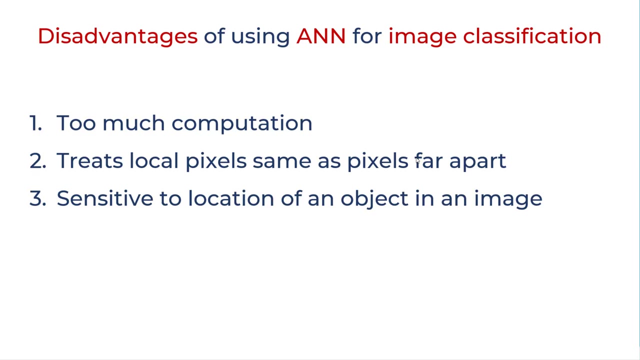 into like 500 million or 1 million of weights that you have to compute, And that's too much computation for your little computer. See, my rabbits are getting electrical shock because it's just too much to do So. the disadvantages of using ANN or artificial neural network for image classification is: 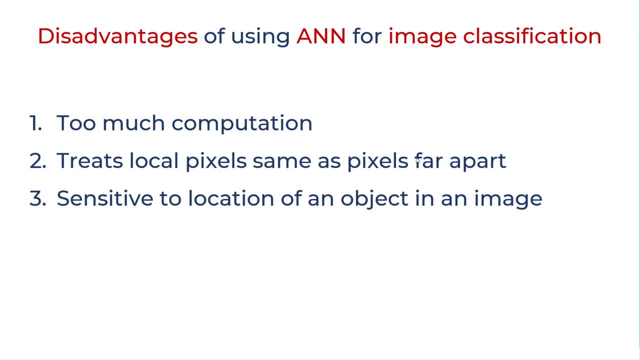 too much computation. It also treats local pixels same as pixels, far apart. If you have koala's face in a left corner versus right corner, it is still a koala, Doesn't matter where the face is located. So the image recognition task is centered around the locality. 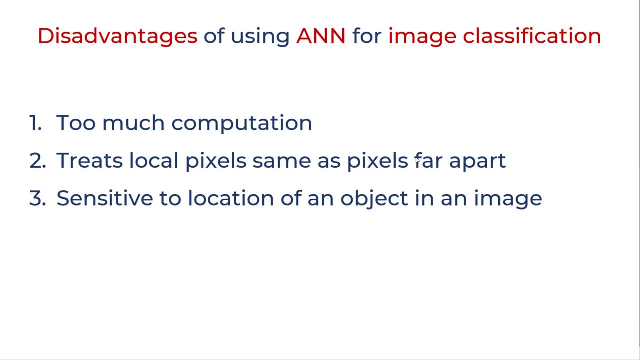 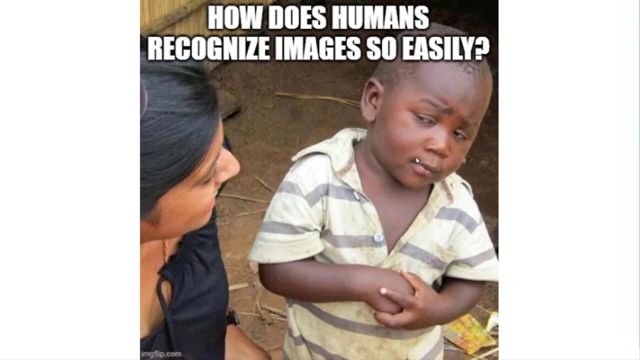 Okay. So if the pixels are moved around, it should still be able to detect the object in an image, But with ANN it's hard. So how does human recognize this image so easily? So let's go into the neuroscience a little bit and try to see how we, as humans, recognize. 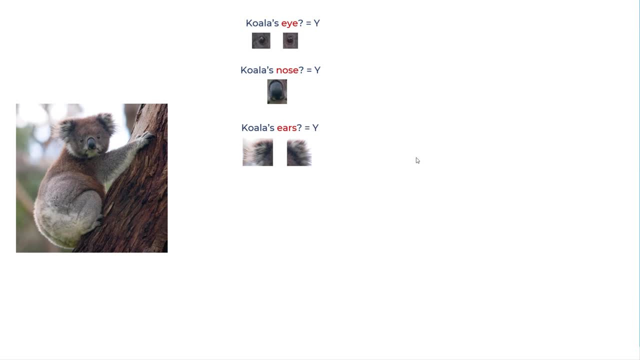 any image so easily. When we look at koala's image, we look at the little features like these round eyes, this black, prominent flat nose, this fluffy ears, and we detect these features one by one In our brain. there are different set of neurons working on these. 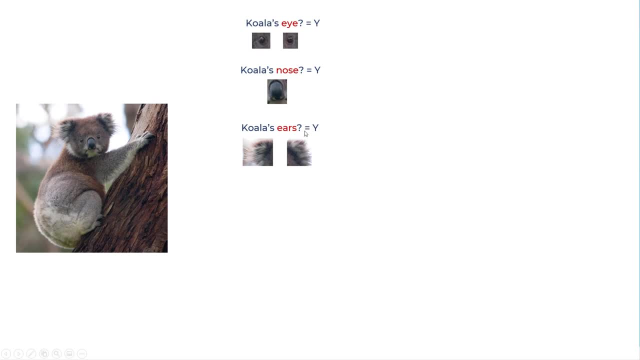 different features and they are firing. They are saying: yeah, I found koala's ears, Yes, I found koala's nose, and so on. Then these neurons are connected to another set of neurons which aggregate the results. It will say: if in the image you are seeing koala's eye, nose, 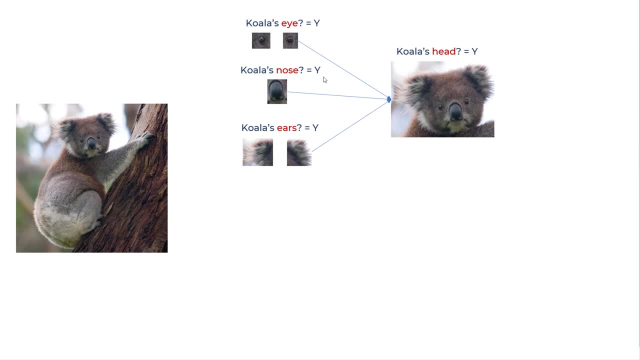 and ears, it means there is a koala's face in the image. Similarly, if there is koala's hands and legs, it means there is koala's body And there are different set of neurons which are connected to these neurons, which will again aggregate the results, saying that if 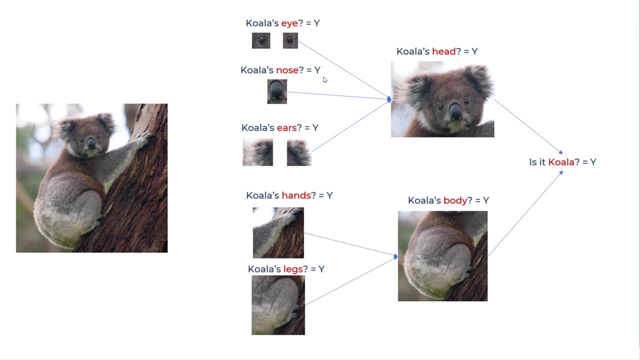 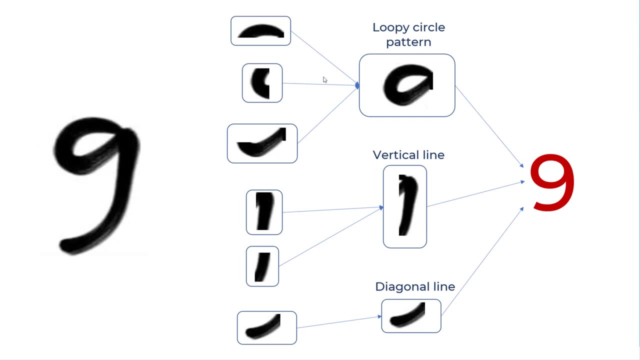 the image has koala's head and body. it means it is koala's image. Same thing with handwritten digit 9.. There are these little edges which come together and form a loopy circle pattern which is kind of like a head of digit 9.. In the middle you: 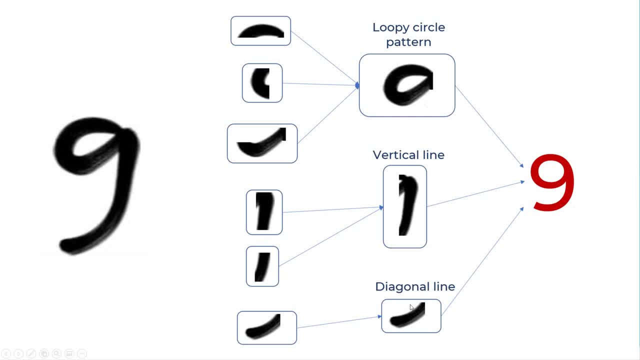 have a vertical line, At the bottom you have diagonal line. Sometimes you don't have diagonal line at all, But we know that whenever there is a loopy circle pattern at the top vertical line, in the middle diagonal line, in the middle vertical line, in the middle diagonal line, 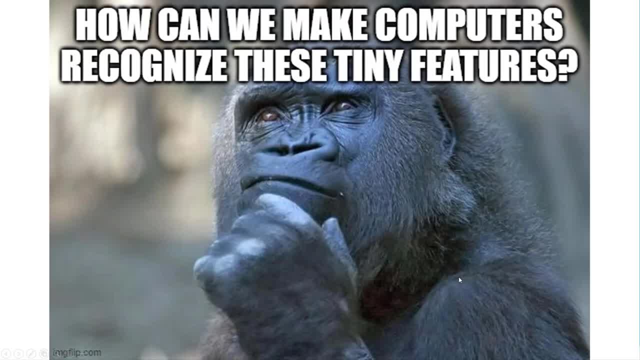 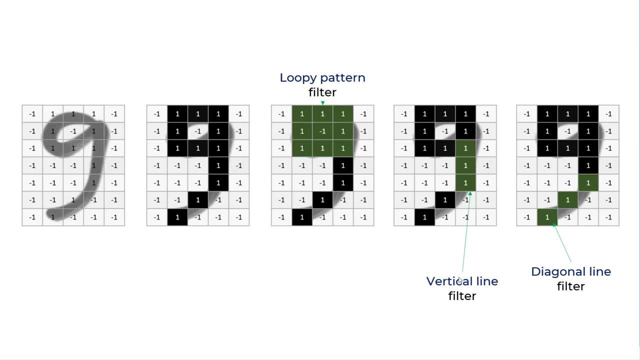 in the end that means digit 9.. So how can we make computers recognize these tiny features? We use the concept of filter. In case of 9, we have three filters. The first one is the head, which is a loopy circle pattern. 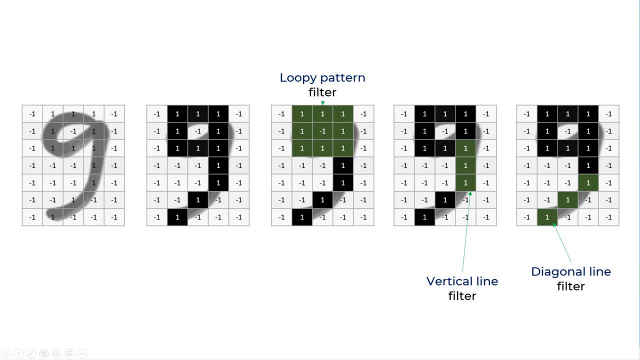 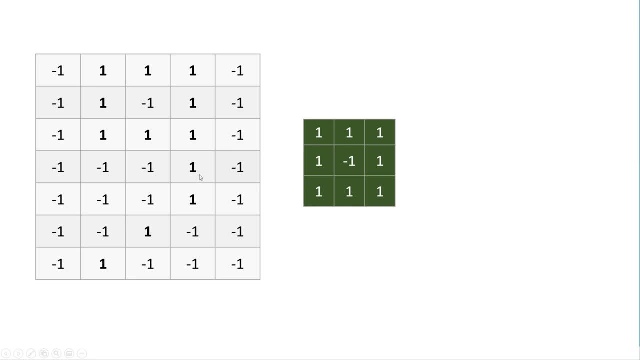 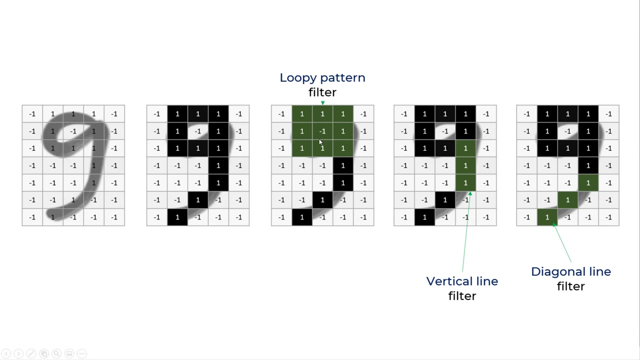 In the middle you have vertical line. In the end you have diagonal filter. We take our original image and we will apply a convolution operation or a filter operation. Here I have a loopy circle pattern or a head filter. This filter right here. 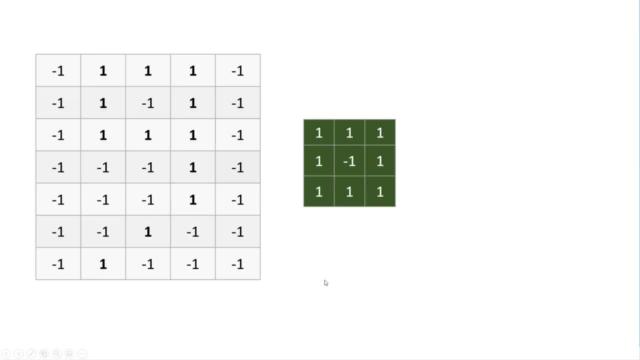 The way convolution operation works is you take 3 by 3 grid from your original image and multiply individual with this filter. so this minus 1 is multiplied with this one, this one is multiplied with this one, and so on. in the end you get a result, and then you 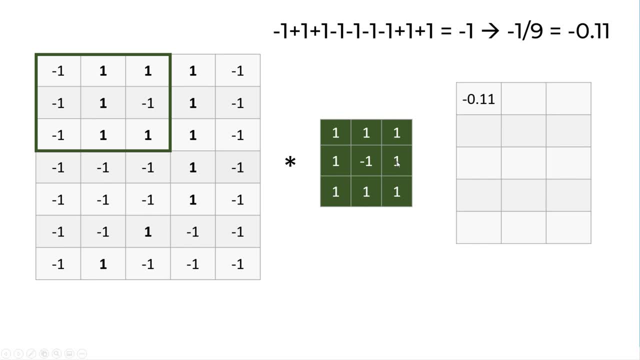 find the average which is divided by 9, because there are total 9 numbers and whatever number you get, you put it here. now this particular thing is called a feature map. so by doing this convolution operation you are creating a feature map. so you do it for the second round of 3 by 3 grid. here I'm taking a stride of 1. 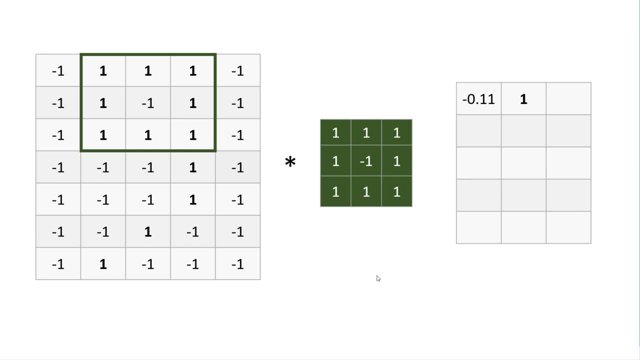 you can take a stride of 2 or 3. also, you don't need to have 3 by 3 filter. you can have 4 by 4 or 5 by 5 filter, and then you keep on doing this for your entire number and in the end, what you get is called a feature map. 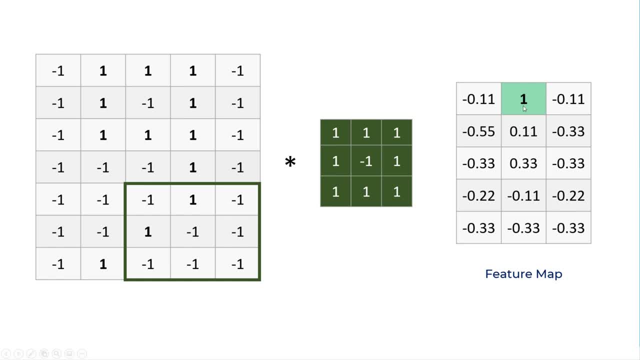 now, the benefit here is, wherever you see number 1 or a number that is close to 1, it means you have a loopy circle pattern. so this is detecting a feature. in the case of koala, this will be eye or a nose, because for koala eye, nose, ears are the 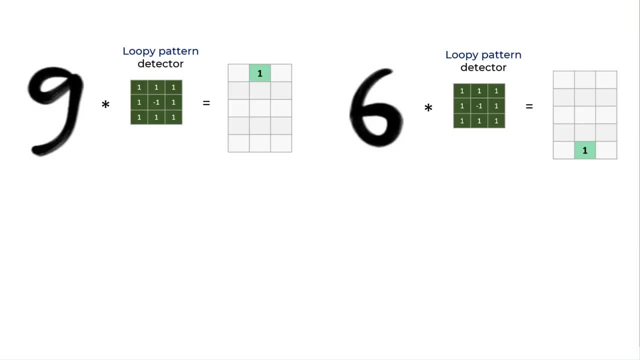 features. so by applying loopy pattern detector I got this one here in my feature map. I also call it. the feature is activated. it got activated here for number 6. it will be activated in the bottom in this area. if you have two loopy patterns, the feature will be activated at top and 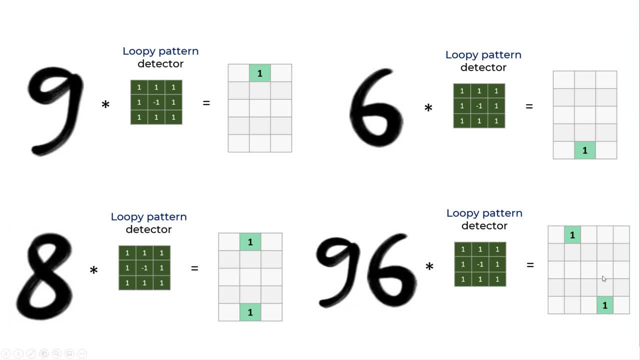 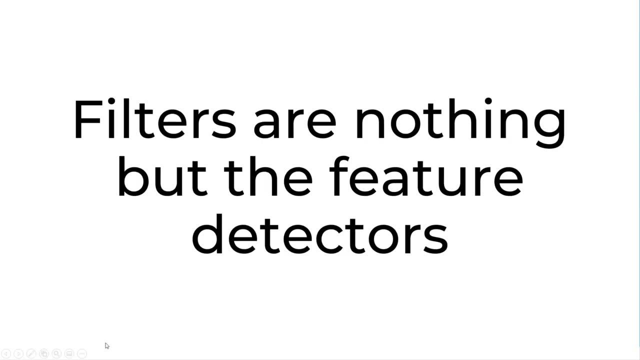 bottom. if your number like this, it might be activated in different area. in summary, when you apply this filter or a convolution operation, you are generating a feature map that has that particular feature detected. so, in a way, filters are nothing but the feature detectors for koalas. 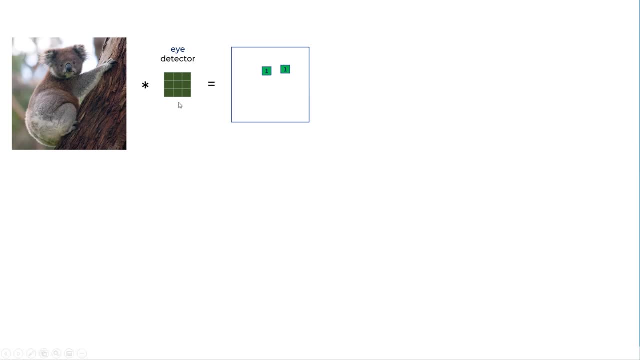 case you can have eye detector and when you apply convolution operation in the result see, you got these two eyes at this location. if the eyes are at a different location, it will still detect, because you are moving the filter throughout the image and they are location invariant, which means doesn't matter where the eyes are. 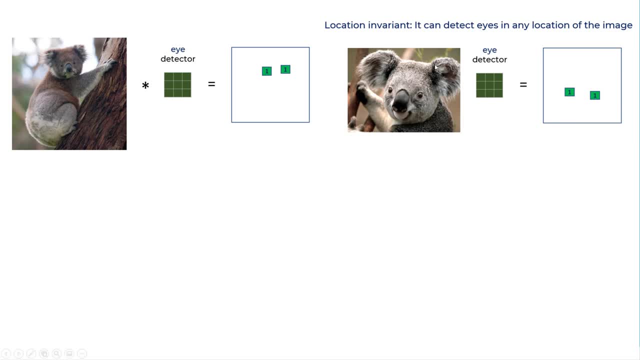 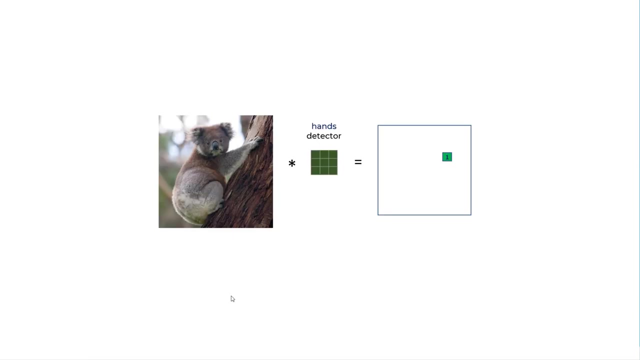 in that location image. these filters will detect those eyes and it will activate those particular regions. here i have six eyes from three different koalas and they are activated accordingly. hooray, the hand of koala is in this particular region for therefore, when i apply hence detector, it will up activate here. 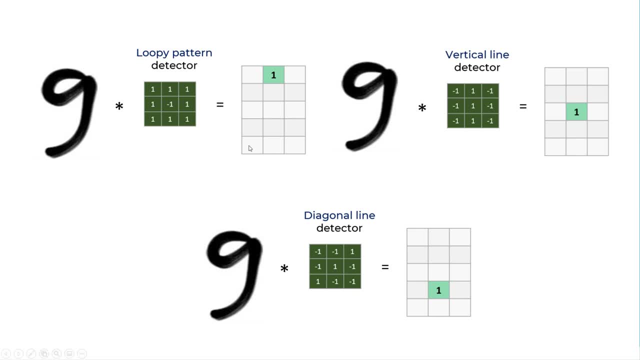 now for number nine, and i'm just moving between number nine and koala so that the presentation is simple enough and you still get an idea. in case of nine, we saw that we need to apply three filters: the head, the middle part and the tail- and when you apply those you get three feature maps. so i applied three filters, i got three. 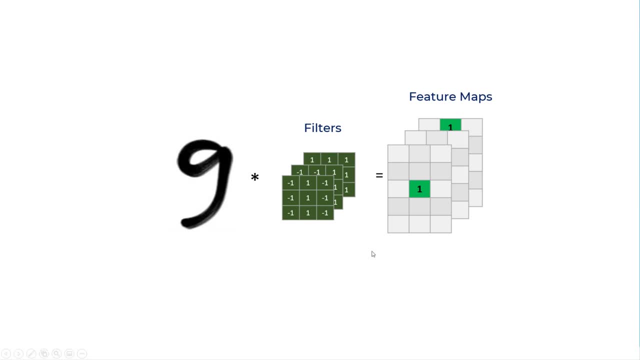 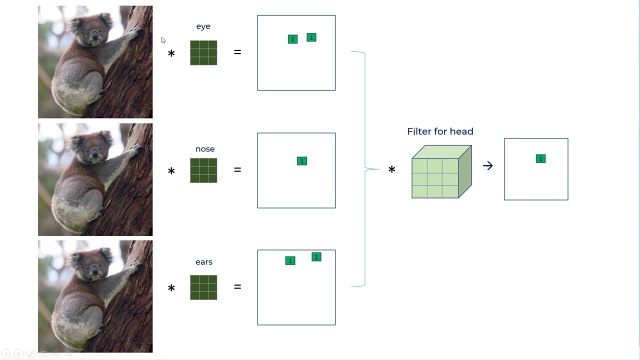 feature maps and this is how these feature maps are represented, represented if you are reading any online article or a book. they are kind of stacked together and they almost form a 3d volume. in case of koala, my eye, nose and ear filters will produce three different feature maps. 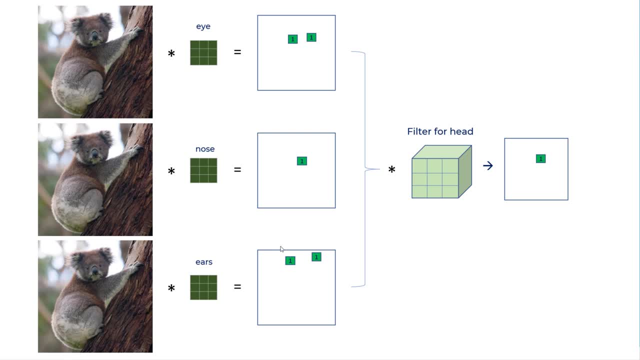 and i can apply convolution operation again, and let's say, this time the filter is to detect head. by the way, the filter doesn't have to be 2d, it can be three-dimensional as well. so just imagine: this first dimension is representing eyes and the second slice is: 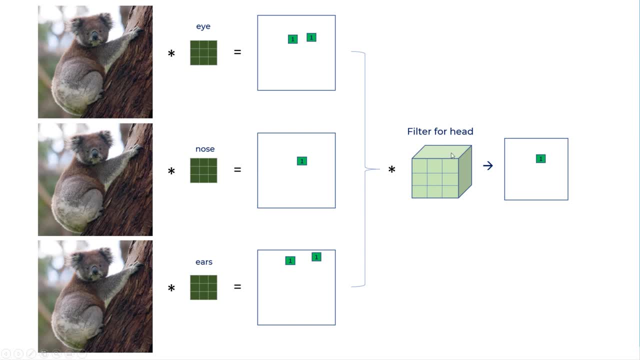 representing nose, and third slice it is representing ears, and by doing that filter you can say that koala's head in is in this particular region of an image. so you are aggregating these results using a different filter for head and now this becomes a koala head detector. 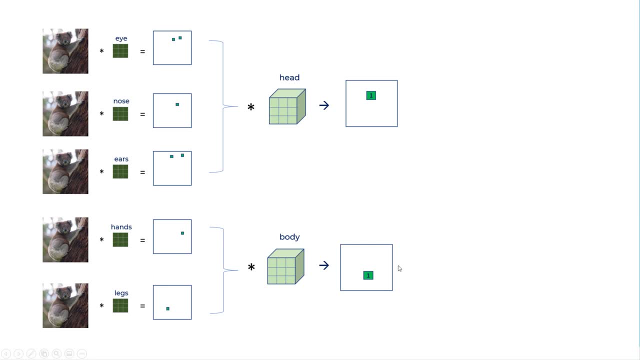 similarly, there could be koala body detector. and now we got these two new feature maps where this feature map is saying that koala's head is at this location and koala's body is at this particular location, then we flatten this number. see, in the end these are like two dimensional numbers. so we 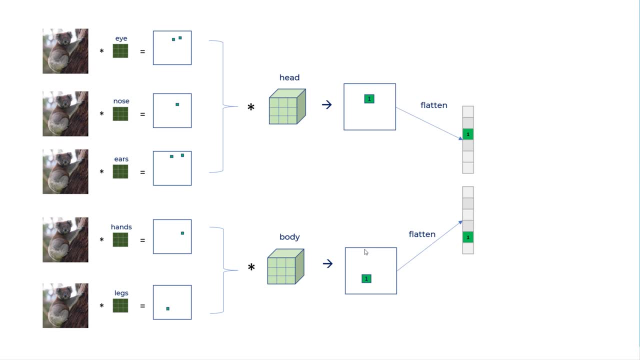 flatten them so to convert 2d array into 1d array and then, when you get these two array, just join them together. after you join, you can make a fully connected dense neural network for your classification. now why do we need this fully connected network here? well, you can have a different image of koala see. 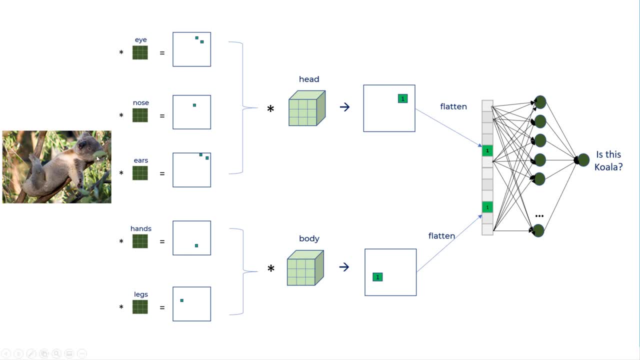 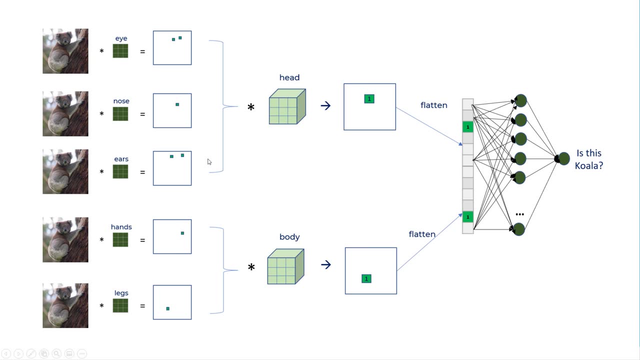 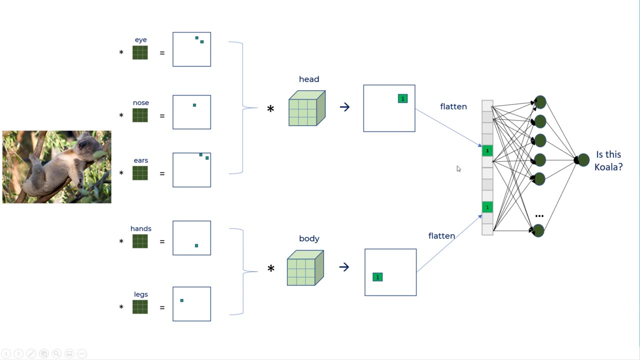 my koala is sleeping. he's tired, so now his eyes and ears are at a different location. look at his ears. see, they're here. for previous image the ears were in a different location, so that generates a different type of flattened array here. and you all know, if you know basics about neural network, that neural 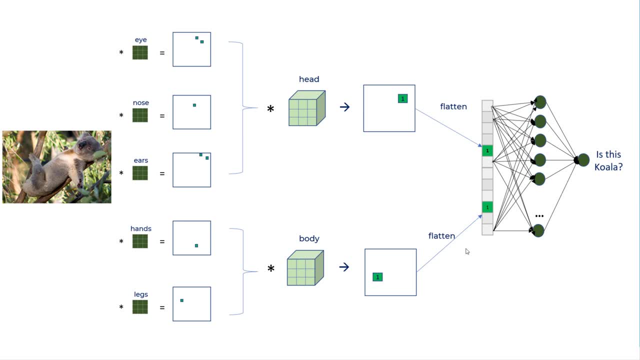 networks are used to handle the variety in neural networks are used to handle the variety in your inputs such that it can classify those variety of inputs in a generic way. here the first part where we use convolutional convolution operation is feature extraction part, and the second portion where we are using dense neural 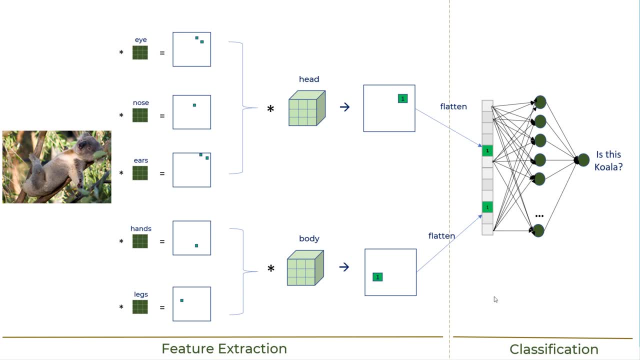 network is called classification, because the first part is detecting all the features- ears, nose, eyes, head and body, etc. and the second part is reception, responsible for classification. we also perform a relu operation, so so this is not a complete convolutional neural network. there are two other components. 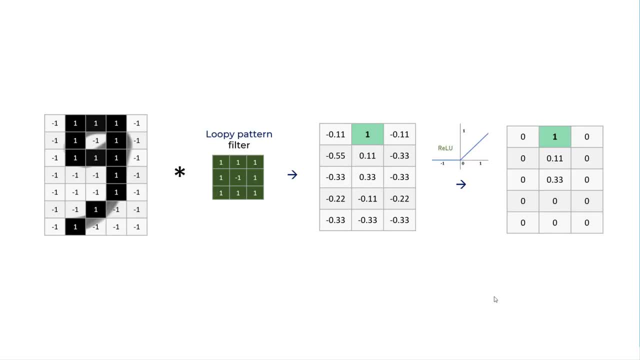 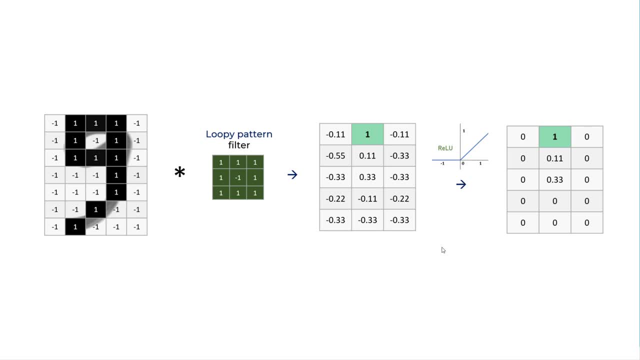 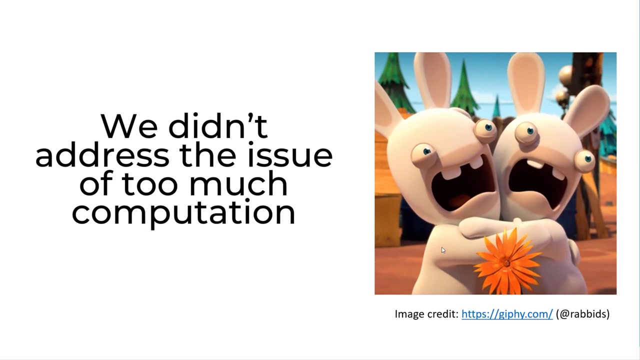 an idea on why it brings the non-linearity especially, see the video on the activations in the same tutorial series, the. the link of this playlist is in the in the video description below, so you'll understand why relu makes it non-linear. but we did not address the issue of too much competition yet. my rabbits are still getting electrical shock. do something, because see for this image size if you are applying. 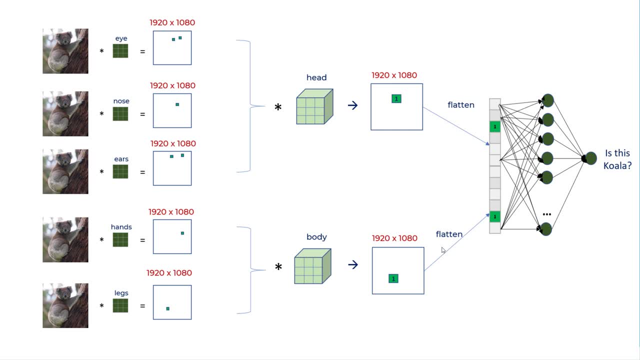 convolution. let's say, with some padding, you're still getting same size of image convolution. let's say, with some padding, you're still getting same size of image convolution. let's say: with some padding, you're still getting same size of image. you did not reduce the image size sometimes. 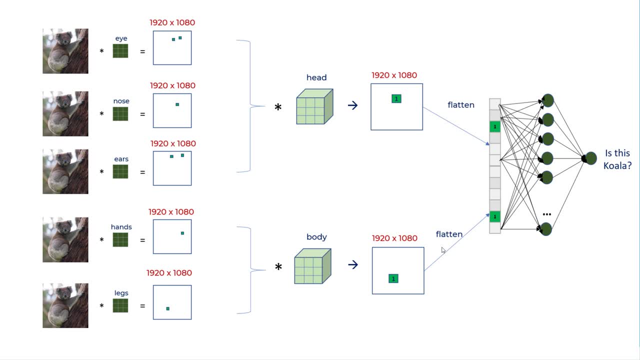 you did not reduce the image size. sometimes you did not reduce the image size. sometimes people don't use padding, so they people don't use padding, so they people don't use padding. so they reduce the image size, but only little bit. so reduce the image size, but only little bit. so. 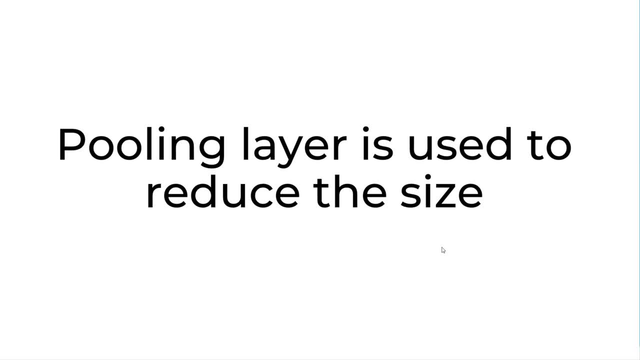 reduce the image size, but only little bit. so pulling is used to reduce the size. the pulling is used to reduce the size. the pulling is used to reduce the size. the main purpose of pulling is to reduce. the main purpose of pulling is to reduce. the main purpose of pulling is to reduce the dimension so that my computer doesn't get. 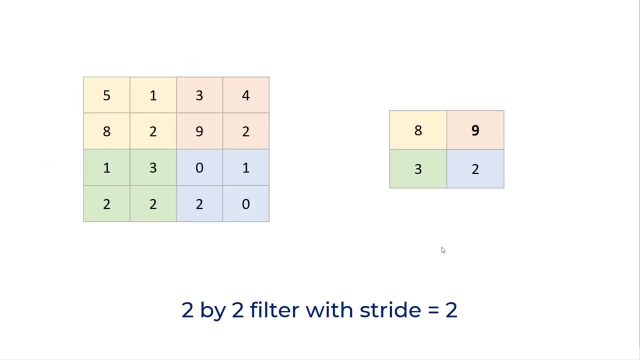 dimension, so that my computer doesn't get dimension, so that my computer doesn't get this shock. you know so, the first, this shock, you know so, the first, this shock, you know so, the first pulling operation is the max pulling, so pulling operation is the max pulling, so 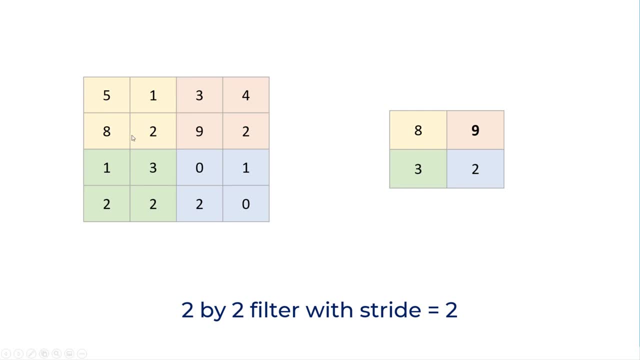 pulling operation is the max pulling. so here you take a window of 2 by 2 and you, here you take a window of 2 by 2 and you, here you take a window of 2 by 2 and you pick the maximum number from that window. 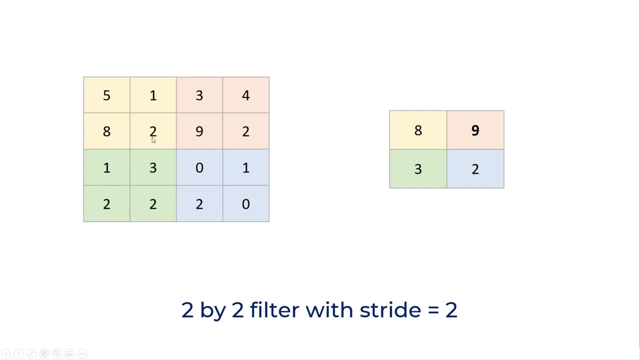 pick the maximum number from that window. pick the maximum number from that window and put it here. so here, check this and put it here. so here, check this and put it here. so here, check this yellow window: 5, 1, 8, 2. what is the? 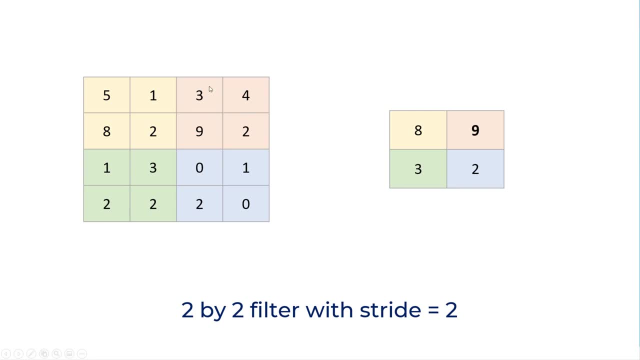 yellow window: 5, 1, 8, 2. what is the yellow window? 5, 1, 8, 2. what is the maximum number? 8, so put 8 here here. maximum number: 8, so put 8 here here. maximum number 8, so put 8 here here. what is the maximum number? 9, so put 9. 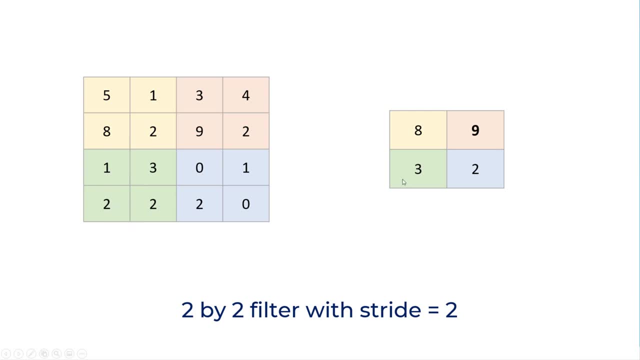 what is the maximum number? 9, so put 9 here. similarly here. maximum number in here, similarly here. maximum number in here, similarly here. maximum number in green window is 3, so put 3, so you take. green window is 3, so put 3, so you take. 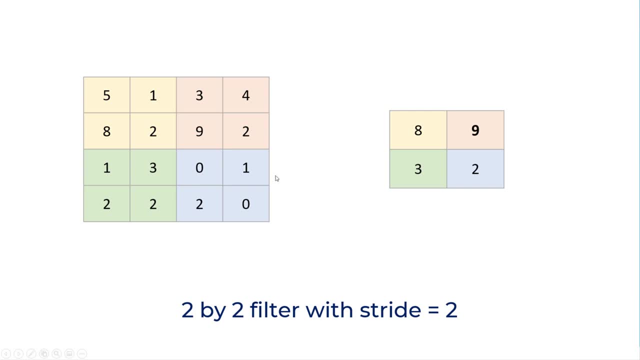 green window is 3, so put 3, so you take the feature map, apply your convoluted the feature map. apply your convoluted the feature map. apply your convoluted. we are pulling and generate a new. we are pulling and generate a new. we are pulling and generate a new feature map after the pulling, but the 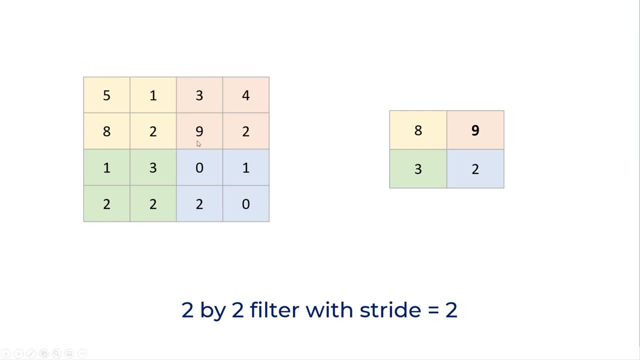 feature map after the pulling. but the feature map after the pulling. but the new feature map is half the size. if you new feature map is half the size. if you new feature map is half the size. if you look at the numbers you know you have. look at the numbers you know you have. 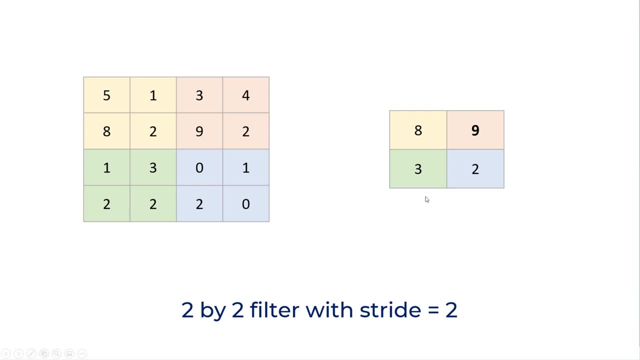 look at the numbers. you know you have reduced your 16 numbers into 4. so it's reduced your 16 numbers into 4. so it's reduced your 16 numbers into 4. so it's too much. or saving in your computation too much, or saving in your computation. 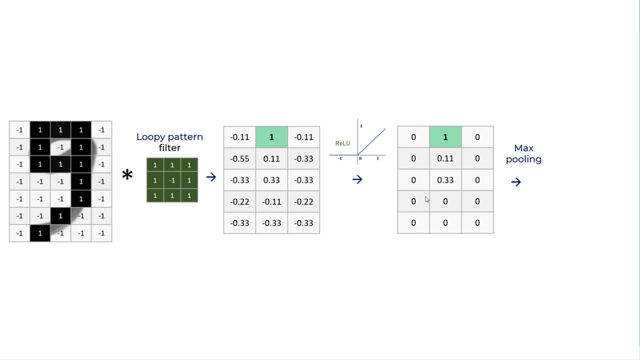 too much or saving in your computation. so how it will look for our digit 9 case. so how it will look for our digit 9 case. so how it will look for our digit 9 case. when you apply max pooling, well you can. when you apply max pooling, well you can. 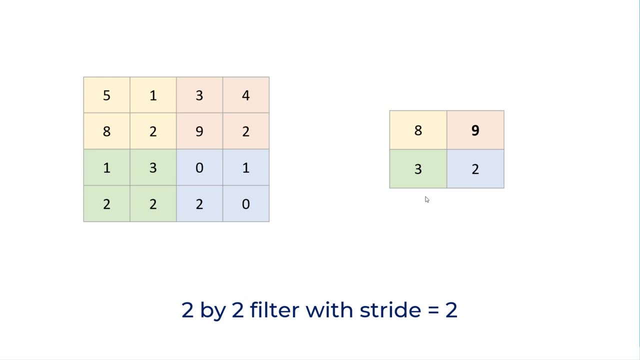 when you apply max pooling. well, you can do a stride of 1- in this case, we did 2- do a stride of 1. in this case, we did 2. do a stride of 1. in this case, we did 2 by 2 window and stride of 2. stride of 2. 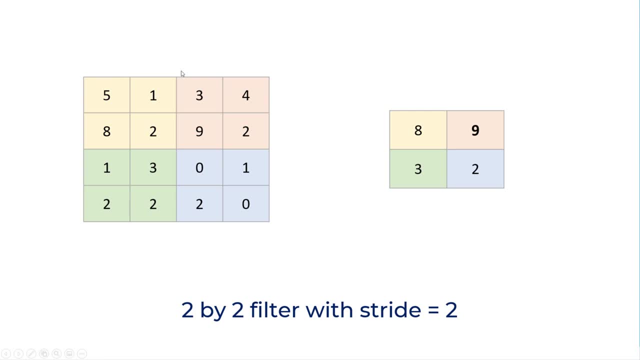 by 2 window and stride of 2. stride of 2 by 2 window and stride of 2. stride of 2 means once we are done with this window. means once we are done with this window. means once we are done with this window, we move two points forward for further. 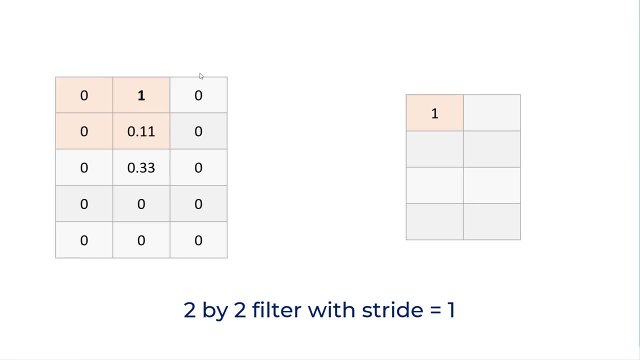 we move two points forward for further. we move two points forward for further. two pixels further. in this case, we can two pixels further. in this case, we can two pixels further. in this case, we can do one stride. see, this is one stride. you do one stride. see, this is one stride. you. 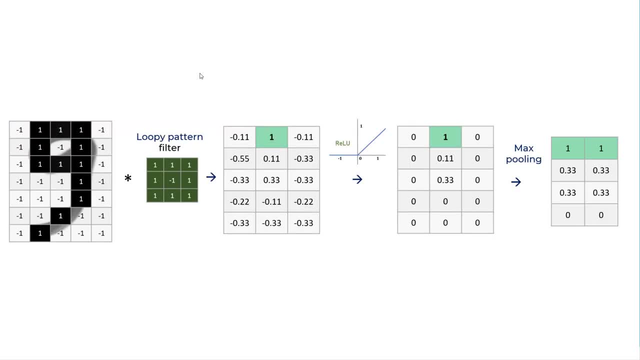 do one stride. see, this is one stride. you get an idea and we keep on taking max. get an idea and we keep on taking max, get an idea and we keep on taking max. and this is what we get when our number, and this is what we get when our number. 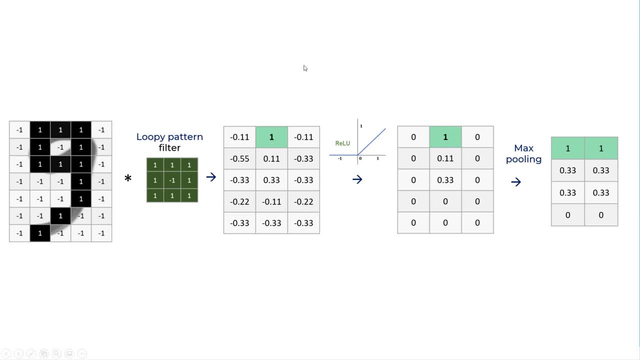 and this is what we get when our number is shifted. so see, this is the original is shifted. so see, this is the original is shifted. so see, this is the original number where we got this max pooling map number, where we got this max pooling map number, where we got this max pooling map. when number is shifted, you get this. 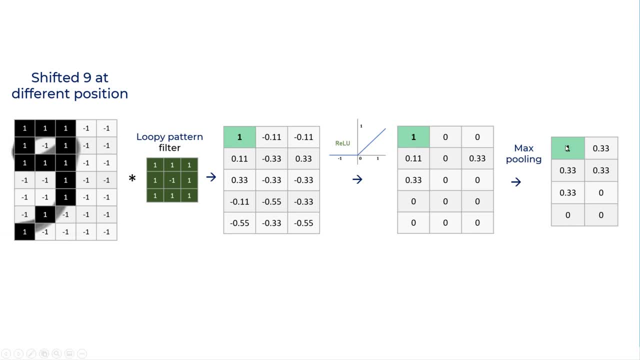 when number is shifted, you get this. when number is shifted, you get this pooling map. so still, you are detecting pooling map, so still, you are detecting pooling map. so still, you are detecting the loopy pattern at the top, so max. the loopy pattern at the top, so max. 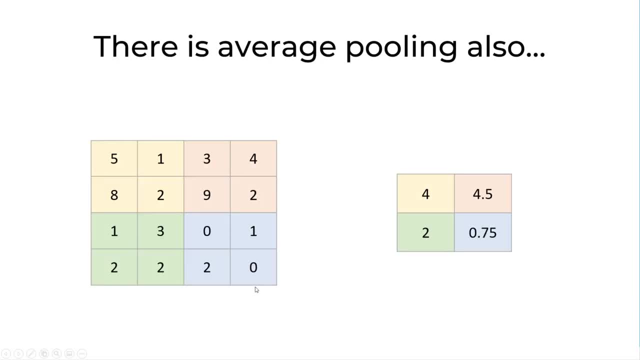 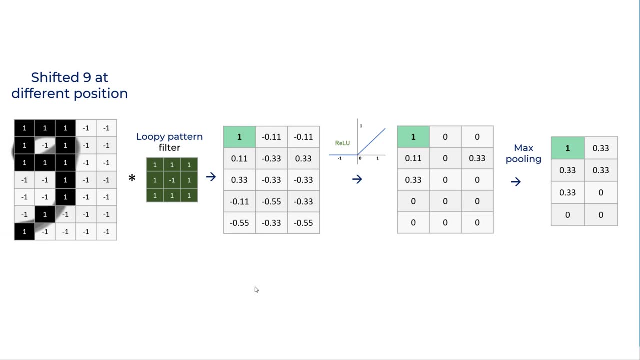 the loopy pattern at the top. so max pulling along with convolution helps you. pulling along with convolution helps you. pulling along with convolution helps you with our position. invariant feature: with our position. invariant feature: with our position. invariant feature. detection doesn't matter where your eyes. detection doesn't matter where your eyes. 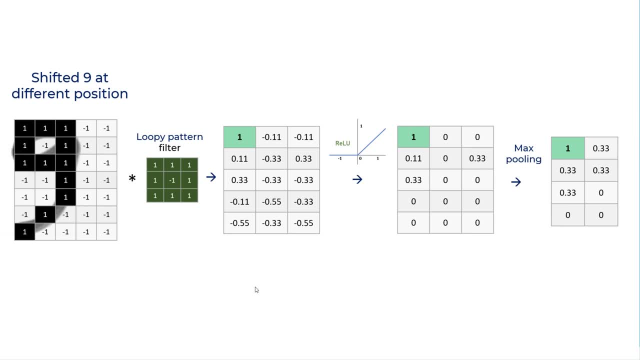 detection doesn't matter where your eyes or ears are in the image, it will detect. or ears are in the image, it will detect. or ears are in the image, it will detect. that feature for you, that feature for you, that feature for you. there is, there is. there is average pooling also instead of max. you. 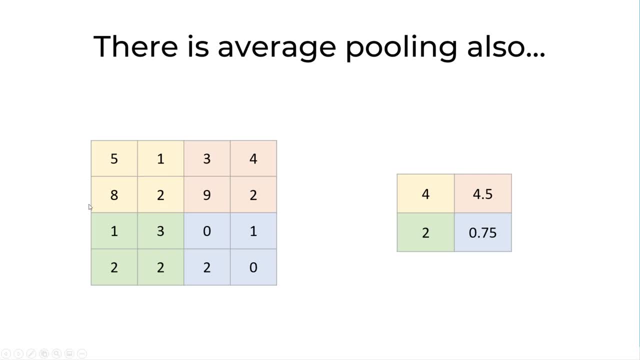 average pooling also instead of max. you average pooling also instead of max. you just make an average: see 5 and 1, 6 and 2. just make an average: see 5 and 1, 6 and 2. just make an average. see 5 and 1, 6 and 2, 8, 8 and 8, 16. 16 divided by 4 is 4, so but 8, 8 and 8, 16, 16 divided by 4 is 4, so but 8, 8 and 8, 16, 16 divided by 4 is 4, so but max pooling is more generally used. but max pooling is more generally used, but 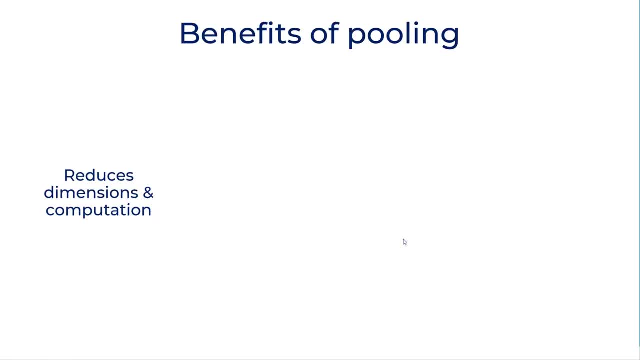 max pooling is more generally used, but sometimes people use average pooling, sometimes people use average pooling, sometimes people use average pooling also also. also. so benefits of pooling number one. so benefits of pooling number one. so benefits of pooling number one: obvious it's reducing your dimension and obvious it's reducing your dimension. and 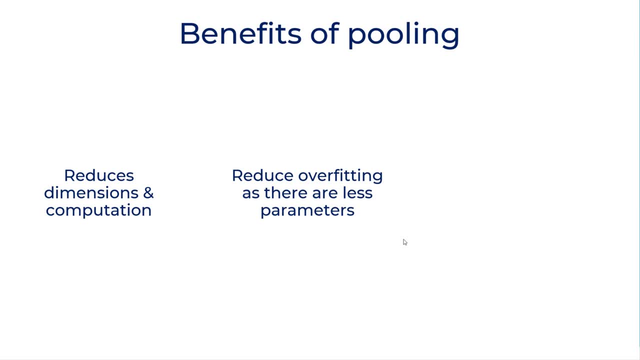 obvious: it's reducing your dimension and computation. the second benefit it computation. the second benefit it computation. the second benefit: it reduce overfitting, because there are less reduce overfitting because there are less reduce overfitting because there are less parameters. and the third one is model. 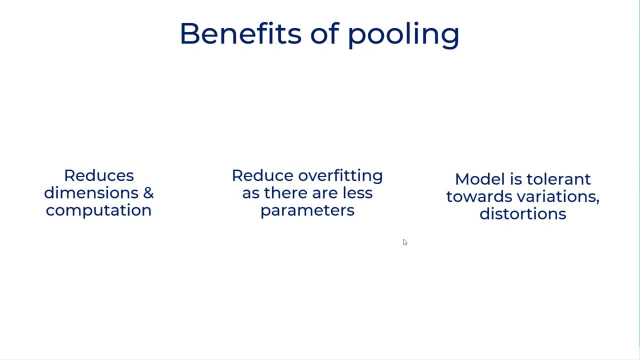 parameters and the third one is model parameters and the third one is model. is variant tolerant towards variation and is variant tolerant towards variation and is variant tolerant towards variation and distortion, because if there is a distortion, because if there is a distortion, because if there is a distortion and if you're picking just a, 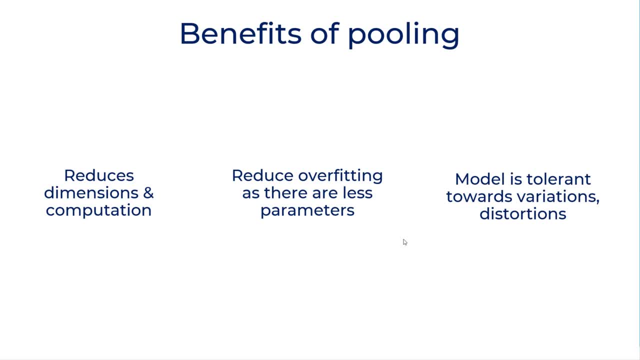 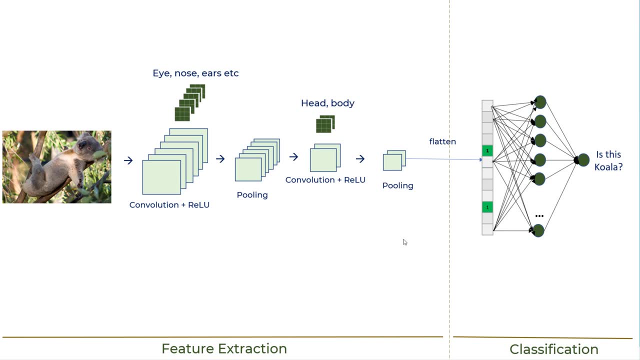 distortion. and if you're picking just a distortion, and if you're picking just a maximum number, you are capturing the maximum number, you are capturing the maximum number, you are capturing the main feature and you are filtering all the main feature. and you are filtering all the main feature and you are filtering all the noise. so this is how our complete 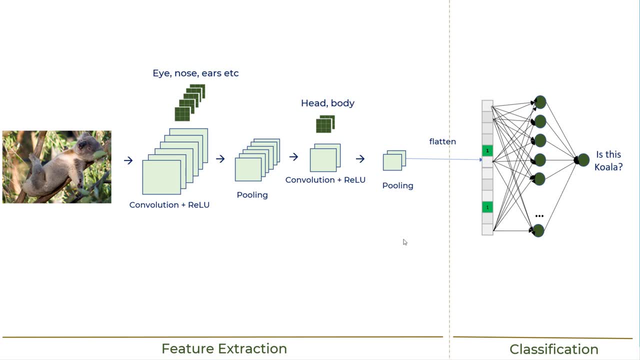 noise. so this is how our complete noise. so this is how our complete convolutional neural network looks like. convolutional neural network looks like convolutional neural network looks like in that you will have typically a. in that you will have typically a. in that you will have typically a convolution and relu layer. then you will. 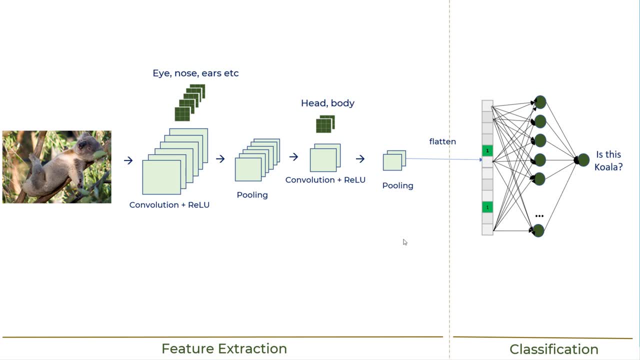 convolution and relu layer, then you will convolution and relu layer, then you will have pulling, then there will be another have pulling, then there will be another have pulling, then there will be another convolution value pulling. there could be convolution value pulling. there could be convolution value pulling. there could be n number of layers for convolution and. 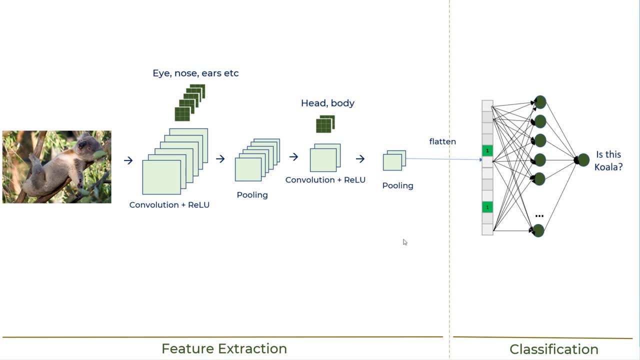 n number of layers for convolution and n number of layers for convolution and pulling, and in the end you will have pulling and in the end you will have pulling and in the end you will have fully connected dense neural network in fully connected dense neural network, in fully connected dense neural network. in this particular case, the first, 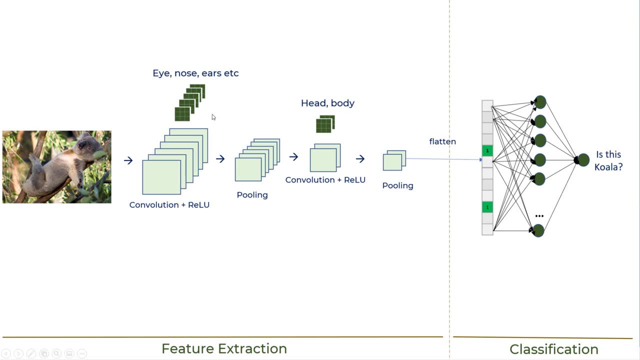 this particular case, the first. this particular case, the first convolution layer is detecting eye nose convolution layer is detecting eye nose convolution layer is detecting eye, nose and ears. many times you will start with and ears. many times you will start with and ears. many times you will start with the little edges. you don't even start. 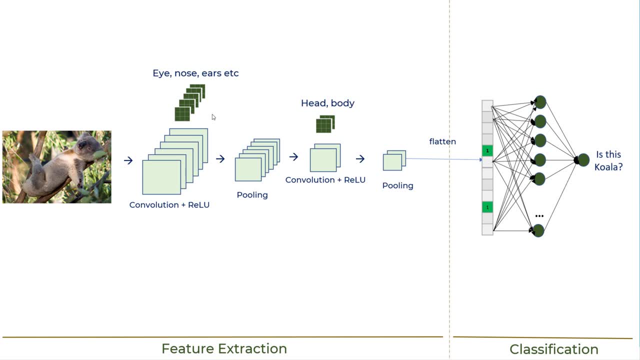 the little edges. you don't even start the little edges. you don't even start with iron nose. but here for the with iron nose, but here for the with iron nose, but here for the simplicity. I have put them, but usually. simplicity I have put them, but usually. 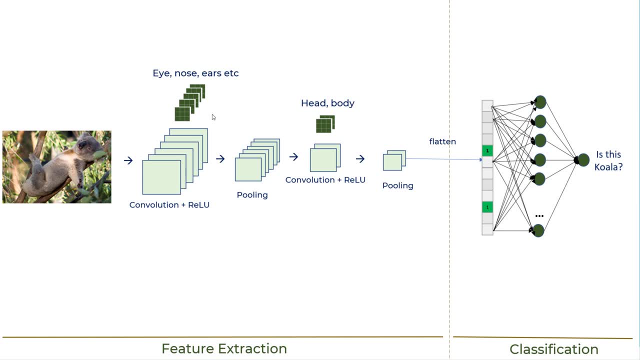 simplicity I have put them, but usually you'll start with edges, then you go to. you'll start with edges, then you go to. you'll start with edges, then you go to eye nose, ears, then you go to head and eye nose ears, then you go to head and 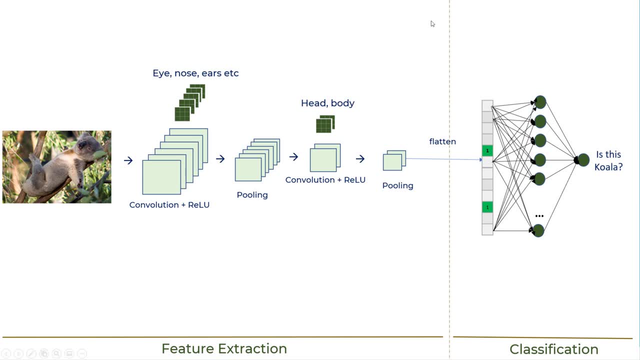 eye, nose, ears. then you go to head and body, and then you do flattening again body, and then you do flattening again body, and then you do flattening again. anything on the left hand side of this, anything on the left hand side of this, anything on the left hand side of this vertical line, is feature extraction. so 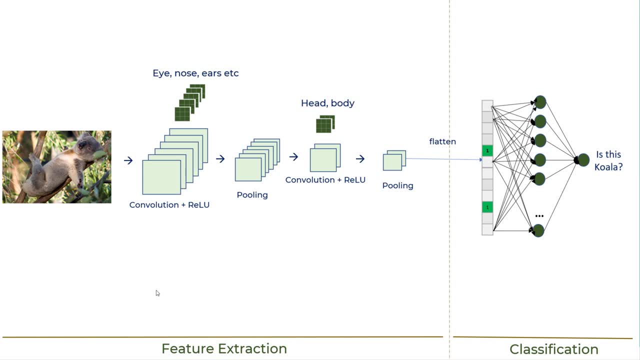 vertical line is feature extraction, so vertical line is feature extraction. so the main idea behind convolutional, the main idea behind convolutional, the main idea behind convolutional neural network is feature extraction. neural network is feature extraction. neural network is feature extraction, because the second part is same. it is a 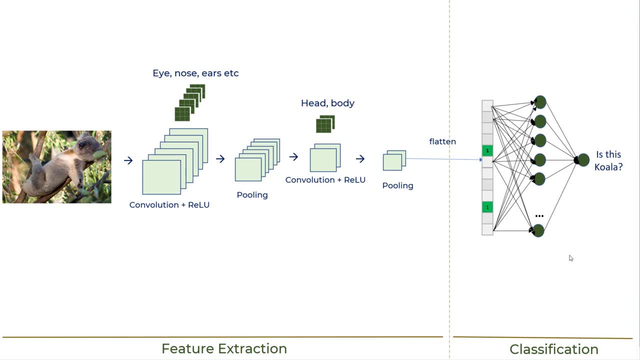 because the second part is same. it is a. because the second part is same, it is a simple artificial neural network, but by simple artificial neural network, but by simple artificial neural network. but by doing this convolution, you are detecting, doing this convolution, you are detecting, doing this convolution, you are detecting the features. you are also reducing the. 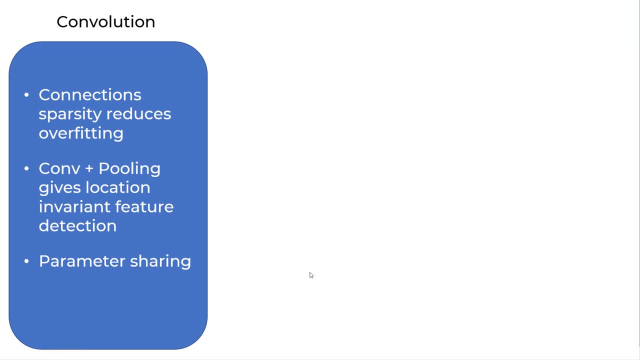 the features. you are also reducing the the features. you are also reducing the dimension. there are three benefits of dimension. there are three benefits of dimension. there are three benefits of convolution operation. the first one is convolution operation. the first one is convolution operation. the first one is connection. sparsity reduces overfitting. 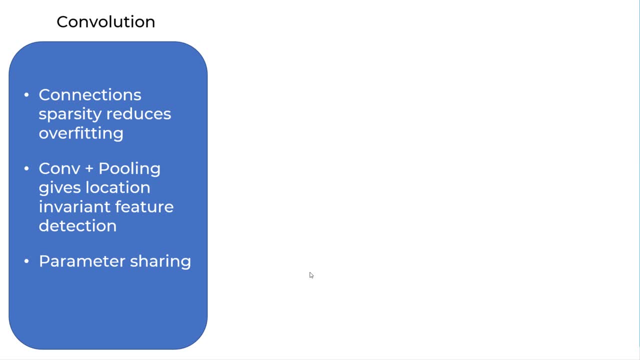 connection sparsity reduces overfitting connection sparsity reduces overfitting connection sparsity means not every node connection sparsity means not every node. connection sparsity means not every node is connected with every other node. like is connected with every other node. like is connected with every other node. like in artificial neural network, where we 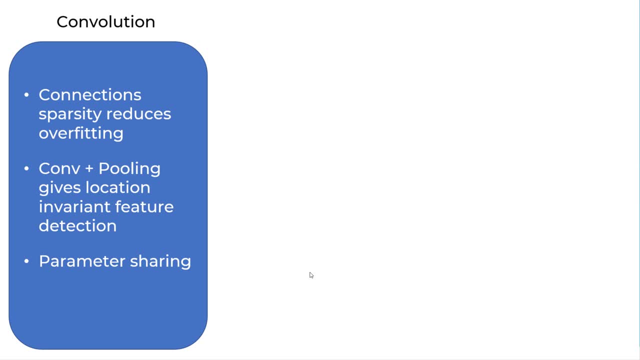 in artificial neural network, where we in artificial neural network, where we call that a dense network, here we have a call that a dense network, here we have a call that a dense network, here we have a filter which we move around the image filter which we move around the image. 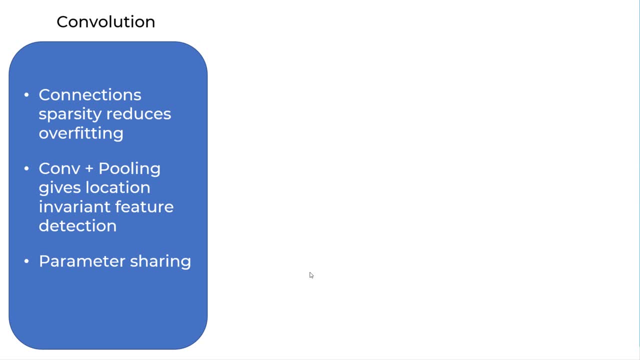 filter, which we move around the image, and at a time we are talking about only a and at a time we are talking about only a and at a time we are talking about only a local region. so we are not affecting local region. so we are not affecting. 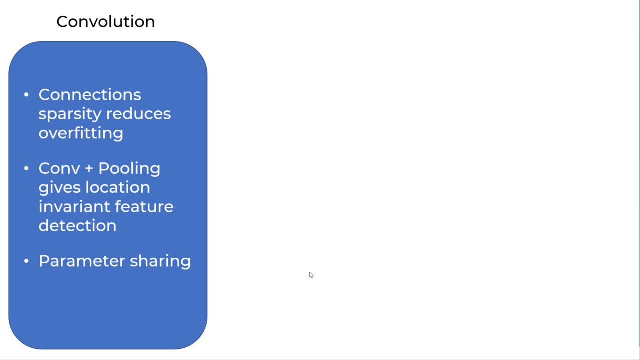 local region, so we are not affecting the whole image. the second benefit is the whole image. the second benefit is the whole image. the second benefit is convolution and pulling operation. convolution and pulling operation. convolution and pulling operation combined gives you a location invariant. combined gives you a location invariant. 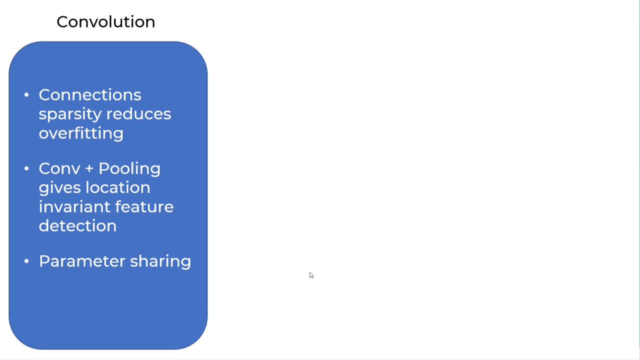 combined gives you a location. invariant feature detection, which means koalas. I feature detection, which means koalas, I feature detection, which means koalas. I could be in the left corner, in the right, could be in the left corner, in the right, could be in the left corner, in the right corner, anywhere. we will still detect it. 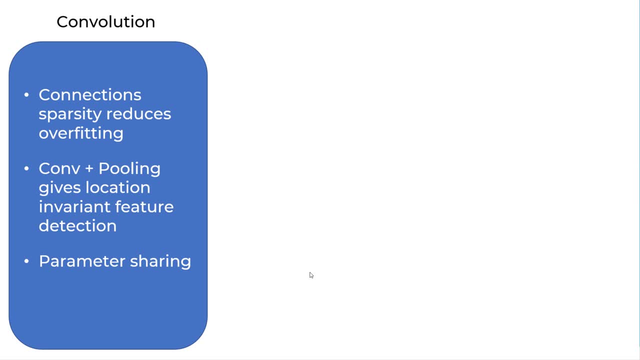 corner anywhere, we will still detect it. corner anywhere, we will still detect it. third is a parameter sharing, which is third is a parameter sharing. which is third is a parameter sharing, which is: when you learn the parameters for a, when you learn the parameters for a, when you learn the parameters for a filter, you can apply them in the entire. 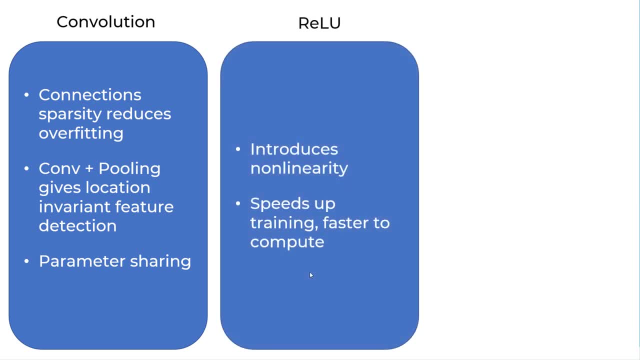 filter. you can apply them in the entire filter. you can apply them in the entire image, image, image. the benefit of value is that it. the benefit of value is that it. the benefit of value is that it introduces non linear linearity, which is introduces non linear linearity, which is. 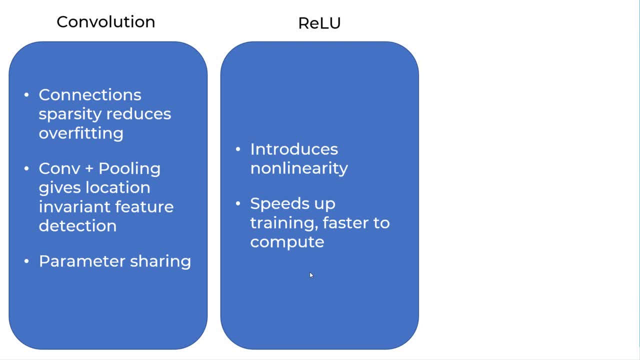 introduces non linear linearity, which is essential because when we are solving a essential, because when we are solving a essential, because when we are solving a deep learning problems, they are non deep learning problems. they are non deep learning problems, they are non linear by nature. it also speeds up. 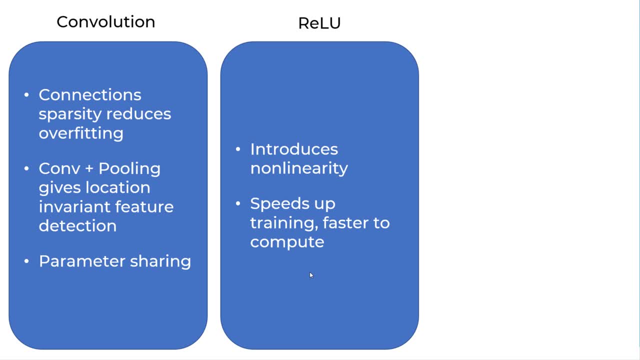 linear by nature. it also speeds up linear by nature. it also speeds up training and it is faster to compute training and it is faster to compute training and it is faster to compute. remember value is you are just doing one. remember value is you are just doing one. 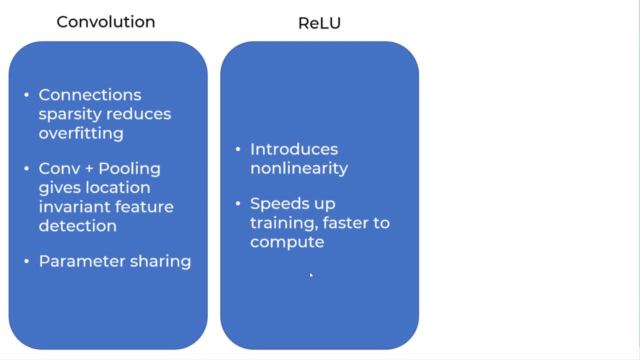 remember value is. you are just doing one: check whether the number is greater. check whether the number is greater. check whether the number is greater than 0 or not. if it is greater than 0 than 0 or not. if it is greater than 0 than 0 or not. if it is greater than 0, keep the number less than 0. make it 0. 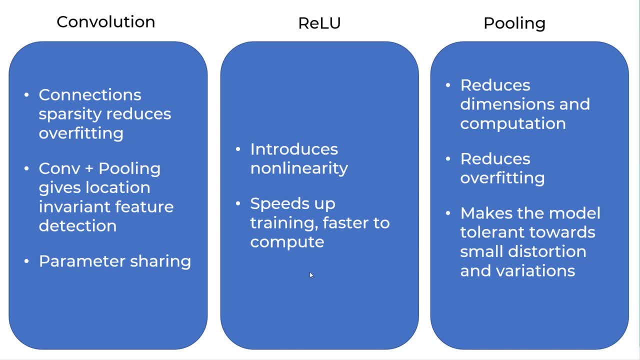 the benefit of pulling is that it. the benefit of pulling is that it. the benefit of pulling is that it reduces dimension and computation. it reduces dimension and computation. it reduces dimension and computation. it reduces overfitting and make the model reduces overfitting and make the model. 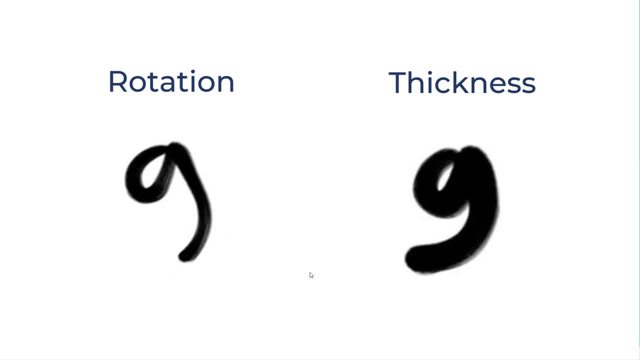 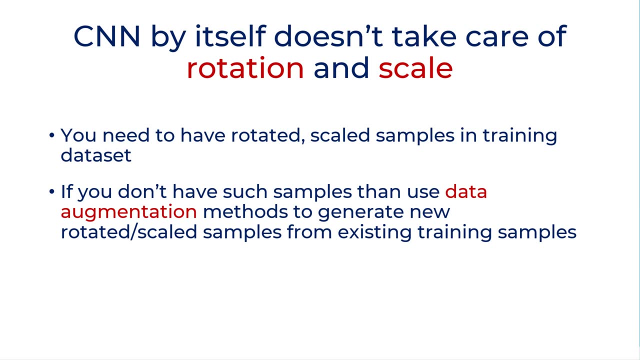 reduces overfitting and make the model tolerant to our small distortions. how tolerant to our small distortions. how tolerant to our small distortions. how about rotation and thickness? because about rotation and thickness? because about rotation and thickness? because by itself the NN cannot handle the 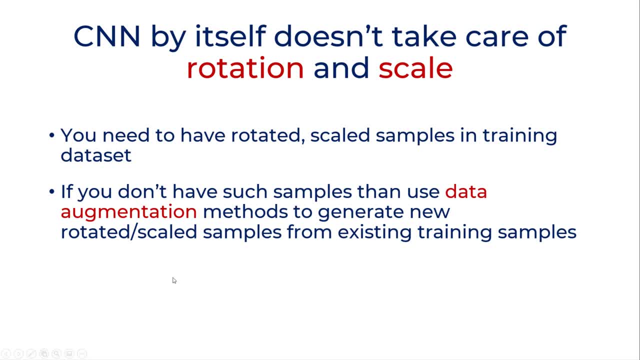 by itself, the NN cannot handle the by itself, the NN cannot handle the rotation, rotation, rotation and the thickness, so you need to have, and the thickness, so you need to have, and the thickness, so you need to have. training samples which have some more, training samples which have some more. 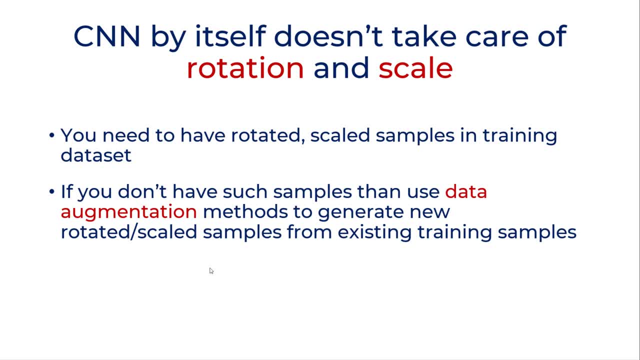 training samples which have some more rotated and scaled sample. you know some rotated and scaled sample. you know some rotated and scaled sample. you know some thick sample, some thin samples and if thick sample, some thin samples and if thick sample, some thin samples, and if you don't, you can use data augmentation. 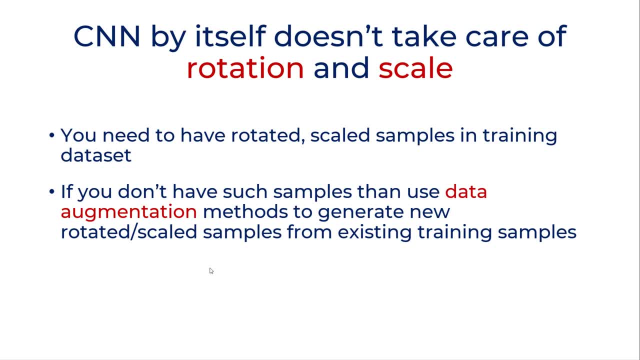 you don't, you can use data augmentation. you don't, you can use data augmentation technique. what is data augmentation technique? what is data augmentation technique? what is data augmentation? let's say for handwritten digits. you, let's say for handwritten digits. you, let's say for handwritten digits, you take your original data set and then you 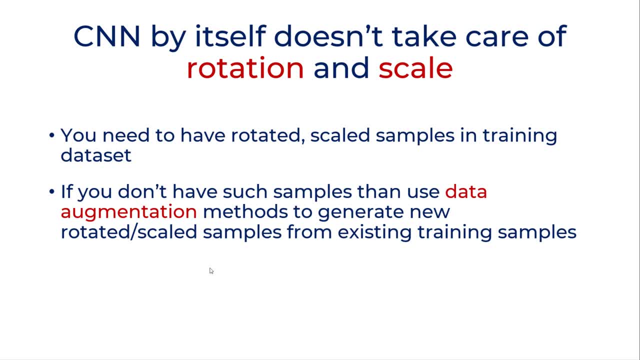 take your original data set. and then you take your original data set and then you pick few samples and then you rotate, pick few samples and then you rotate, pick few samples, and then you rotate them manually, or you make them larger, or them manually, or you make them larger, or 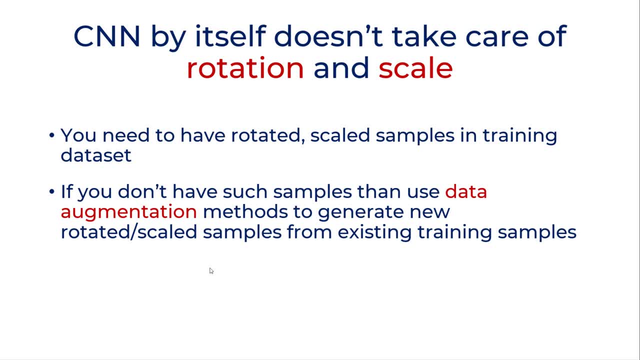 them manually. or you make them larger, or you make them smaller, thicker or thinner. you make them smaller, thicker or thinner. you make them smaller, thicker or thinner. and you generate new samples by doing, and you generate new samples by doing and you generate new samples by doing that. you can handle rotation and scale. 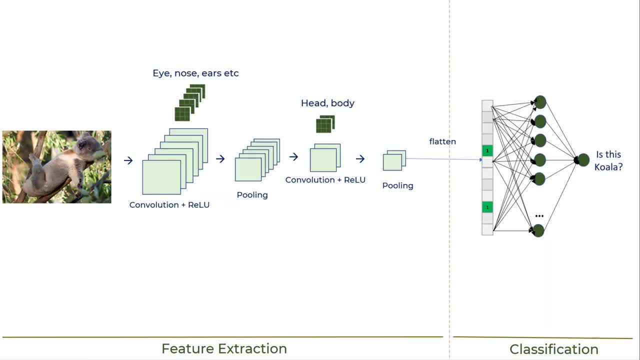 that you can handle rotation and scale, that you can handle rotation and scale in convolutional neural network, in convolutional neural network, in convolutional neural network. once again, here is a quick summary of. once again, here is a quick summary of. once again, here is a quick summary of what is convolutional neural network. you 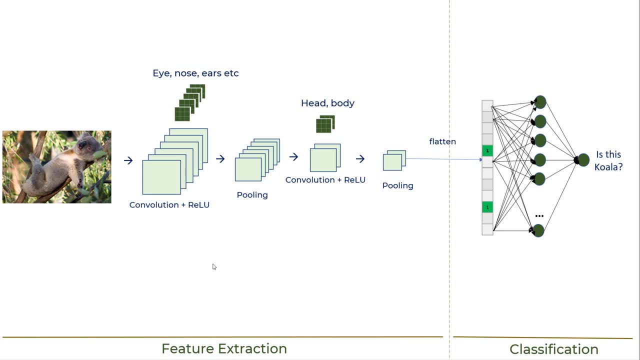 what is convolutional neural network? you what is convolutional neural network? you can take a screenshot of this image. put. can take a screenshot of this image. put. can take a screenshot of this image. put it at your desk if you're trying to it at your desk if you're trying to. 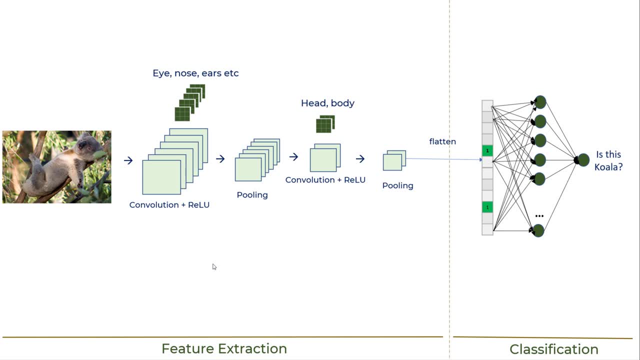 it at your desk if you're trying to learn CNN and a computer vision, to learn CNN and a computer vision, to learn CNN and a computer vision to summarize, you take your input image, then summarize, you take your input image, then summarize, you take your input image, then you apply convolution operation and 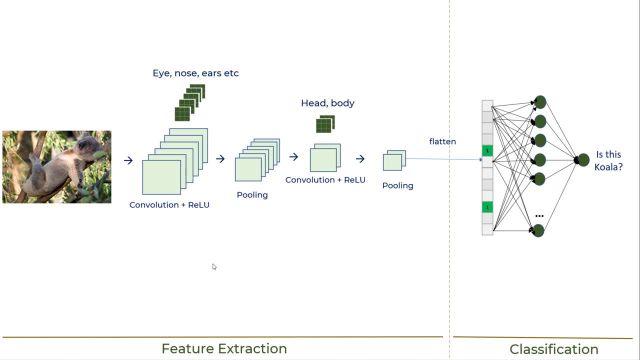 you apply convolution operation. and you apply convolution operation and value, then you apply pulling again value, then you apply pulling again value, then you apply pulling again convolution value pulling, and you can do convolution value pulling and you can do convolution value pulling and you can do this n number of times. after that, the 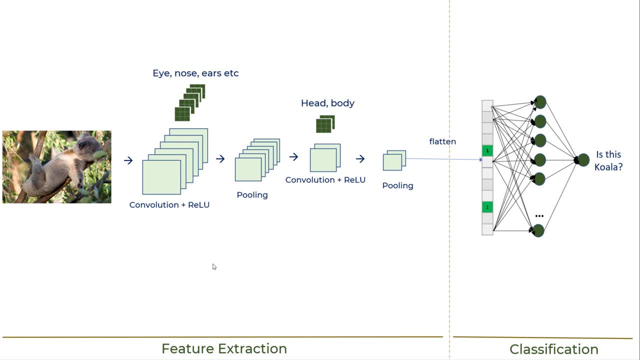 this n number of times. after that the this n number of times after that. the second stage is classification, where you second stage is classification where you second stage is classification where you use densely connected neural network. use densely connected neural network, use densely connected neural network. now, very important thing to mention here: 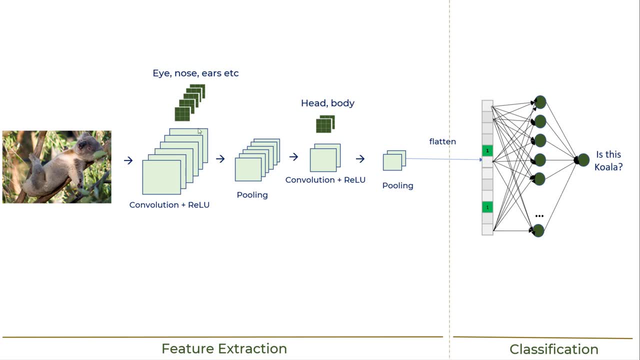 now very important thing to mention here. now very important thing to mention here is these filters the network will learn. is these filters the network will learn. is these filters the network will learn on its own. in previous presentation, we on its own in previous presentation, we on its own in previous presentation, we saw that we applied those filters by 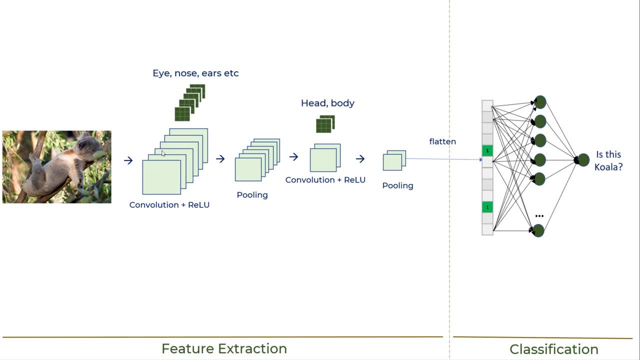 saw that we applied those filters by saw that we applied those filters by hand. but this is the beauty of hand, but this is the beauty of hand, but this is the beauty of convolutional neural network: that it convolutional neural network, that it convolutional neural network, that it will automatically detect these filters on. 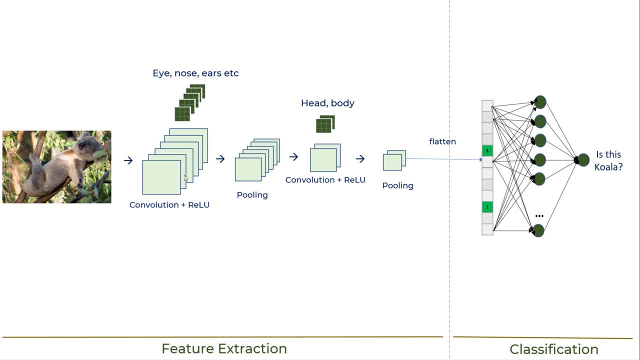 will automatically detect these filters on, will automatically detect these filters on its own, and that is part of the its own, and that is part of the its own and that is part of the training. so when the neural network is training, so when the neural network is training, so when the neural network is training, or when the CNN is training, 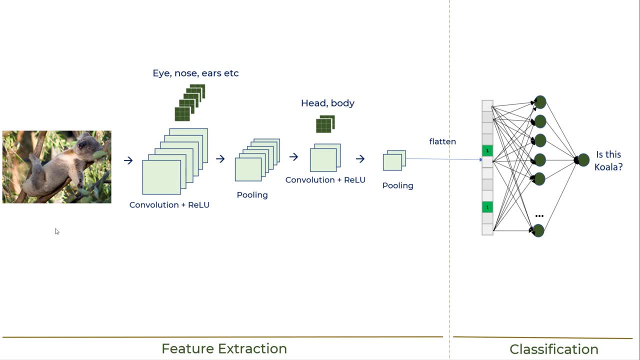 training, or when the CNN is training training, or when the CNN is training, because you're supplying thousands of, because you're supplying thousands of, because you're supplying thousands of koalas images here using that, it will. koalas images here using that, it will. koalas images here using that, it will use back propagation and it will figure. 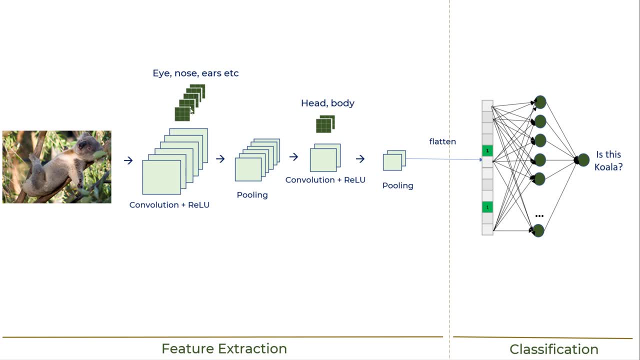 use back propagation and it will figure use back propagation and it will figure out the right amount of filters. it will out the right amount of filters. it will out the right amount of filters. it will figure out the values in this filter and figure out the values in this filter. and. 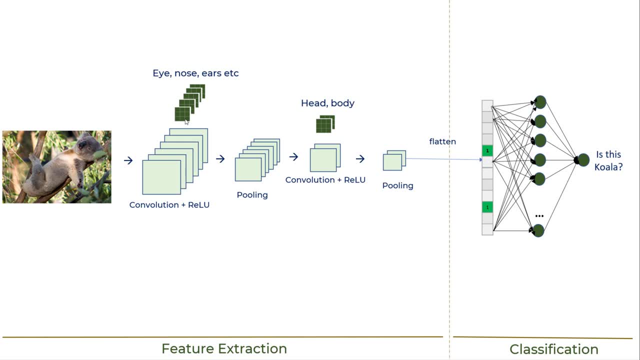 figure out the values in this filter. and that is part of the learning or the back. that is part of the learning or the back. that is part of the learning or the back. propagation as a hyper parameter. you propagation as a hyper parameter. you propagation as a hyper parameter. you will specify how many filters you want to. 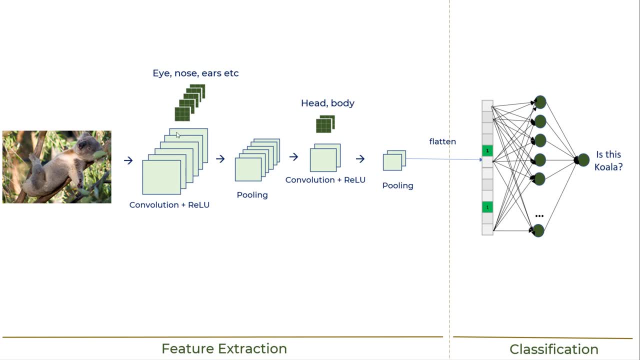 will specify how many filters you want to, will specify how many filters you want to have and what is the size of each of have and what is the size of each of have and what is the size of each of the filters. that's it, but you do not. 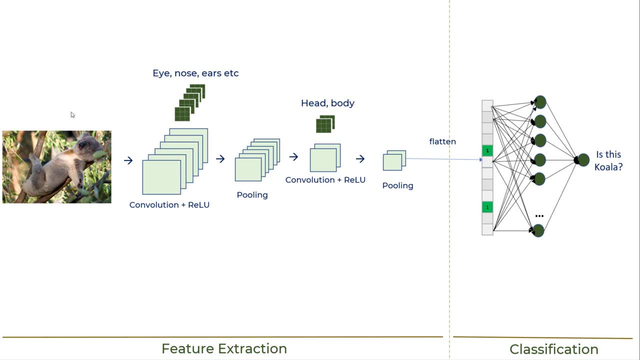 the filters, that's it, but you do not the filters, that's it, but you do not specify the exit values within these. specify the exit values within these. specify the exit values within these filters. the network will learn those on filters. the network will learn those on filters. the network will learn those on its own, and this is that is the most. 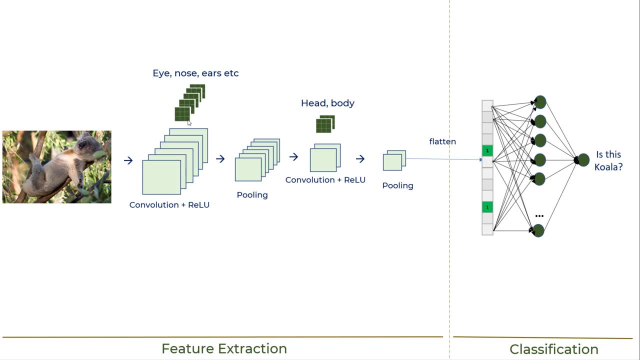 its own and this is that is the most its own and this is that is the most fascinating part about neural network. in fascinating part about neural network, in fascinating part about neural network in general. in next few videos we will be general. in next few videos, we will be. 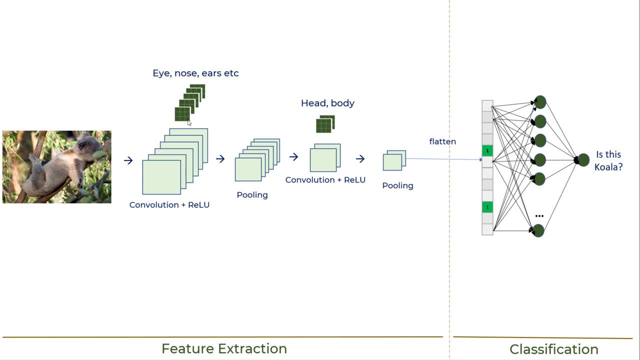 general. in next few videos we will be doing coding using convolutional neural, doing coding using convolutional neural, doing coding using convolutional neural network and will be solving variety of network. and will be solving variety of network and will be solving variety of computer vision problems. so I hope you. 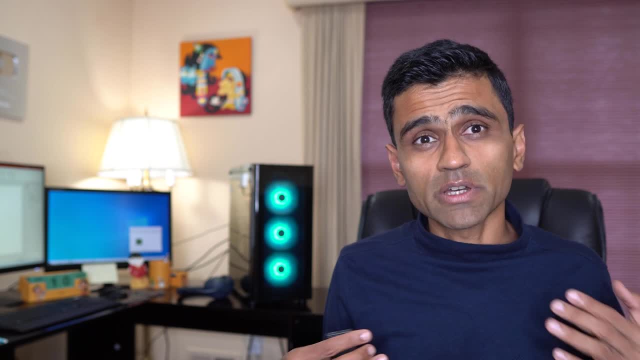 computer vision problems. so I hope you computer vision problems, so I hope you like this explanation. if you don't know, like this explanation. if you don't know, like this explanation. if you don't know me, I'm the world Patel, I teach data me. I'm the world Patel, I teach data. 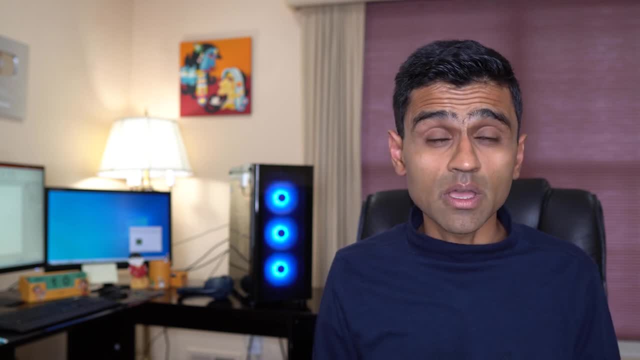 me. I'm the world Patel. I teach data science, machine learning, Python science, machine learning, Python science, machine learning, Python programming and career guidance on my programming and career guidance on my programming and career guidance on my youtube channel. if you are starting youtube channel. if you are starting. 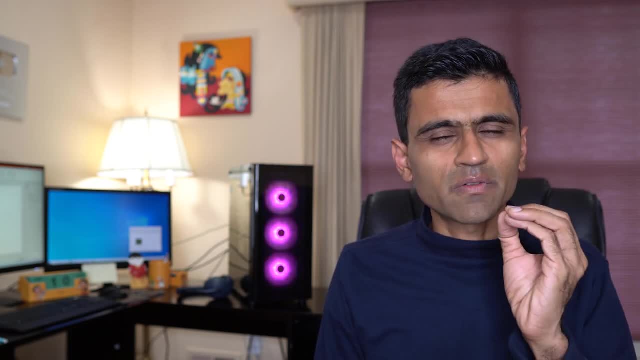 youtube channel. if you are starting, then I have a complete playlist. you can. then I have a complete playlist. you can, then I have a complete playlist. you can start with very basic Python and pandas. start with very basic Python and pandas. start with very basic Python and pandas. knowledge on this playlist and can learn.